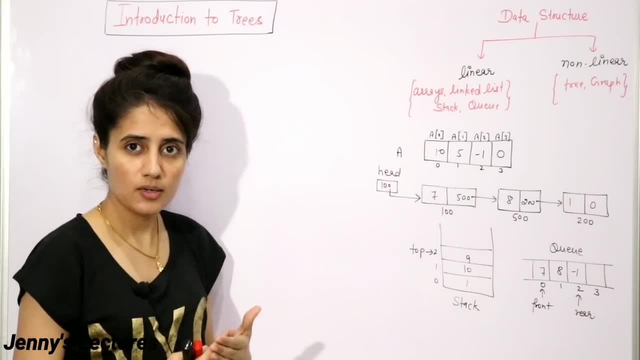 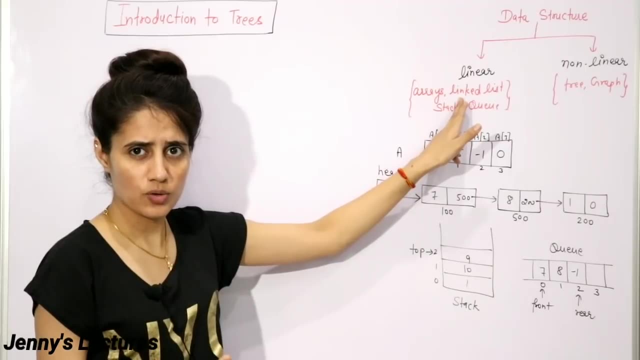 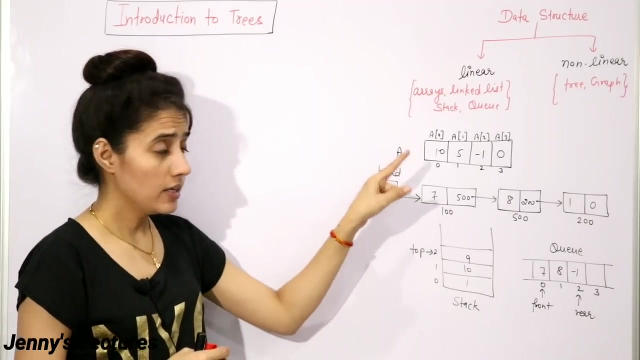 But known linear data structure is having multiple levels, right, The data is stored in sequential manner or which is going to form a special ordering, Some sort of ordering, you can say. But in known linear, the data structure is having multiple levels, right, The data is in the form of hierarchy. you can say, right, The difference between linear 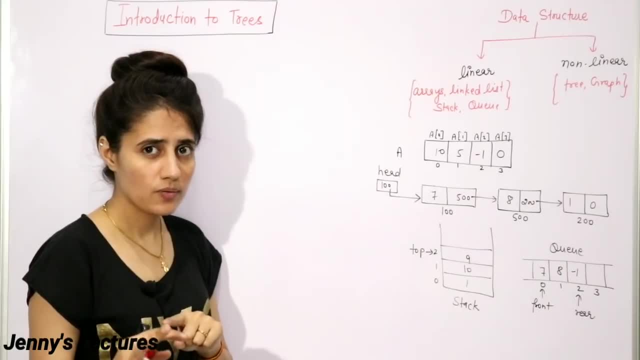 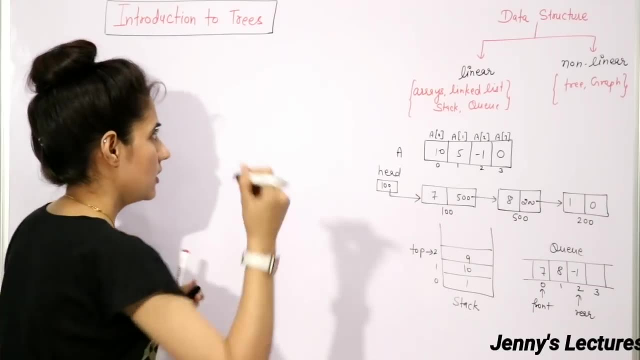 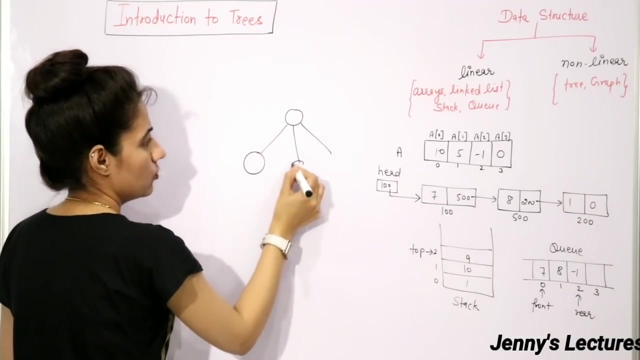 and known linear data structure will discuss in a separate video. right. So now, what is a hierarchical data? You can take an example of a college employees. Fine, see here, at this level maybe you have the director, and below this, three persons are also there. here you. 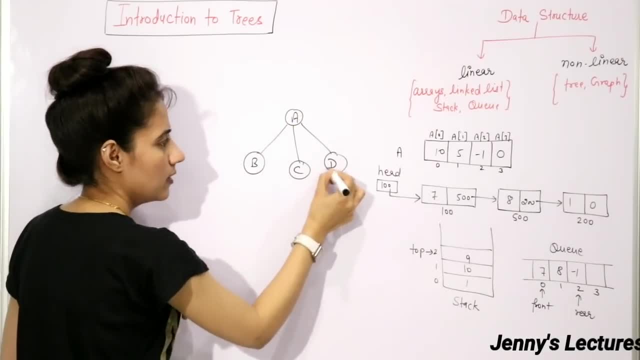 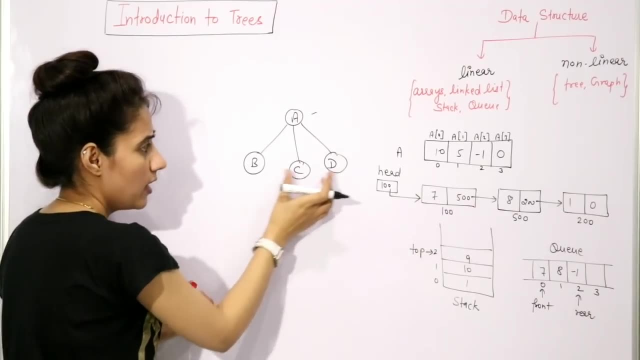 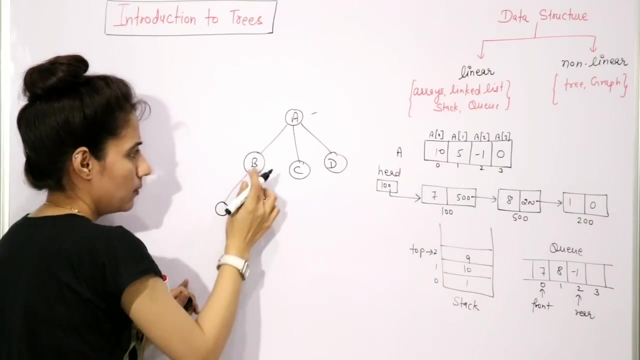 can say A And this one is B, C and D can say this one is maybe director or these are having dean, or principal or something like this. these are going to directly report to the director. below these, maybe we are having below this dean, maybe we are having hods, you can say right, manager, or something like this. if you 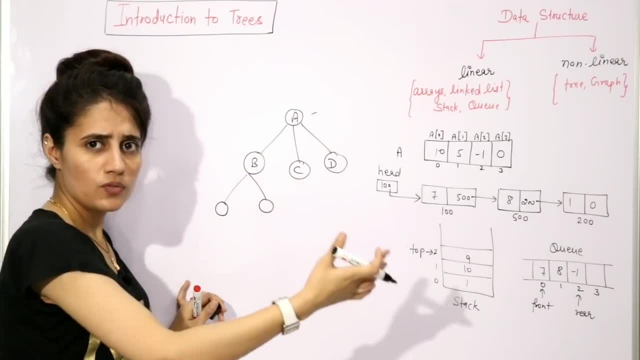 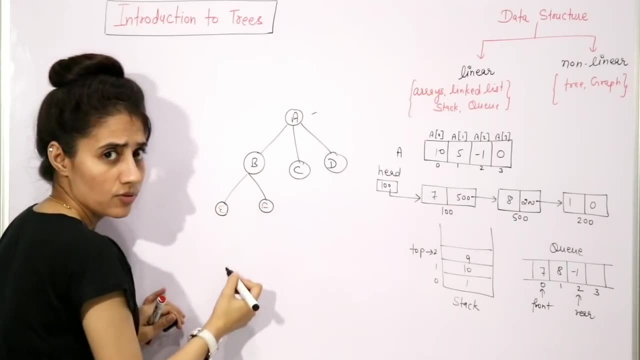 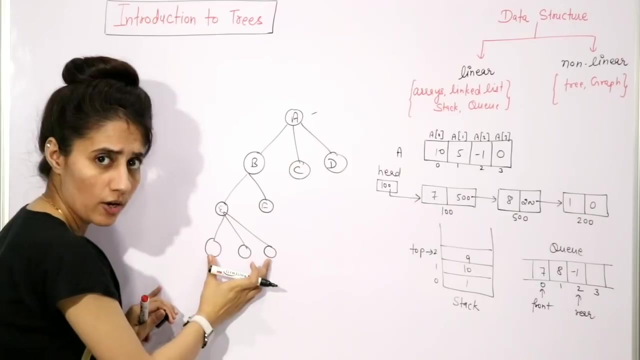 are taking an example of a company. here you can consider ceo of the company manager, assistant manager, team lead and something like this, right? so here you can say e and f below hods. we are having some faculty members, right? so these faculty members are going to report to hod. hod is going to. 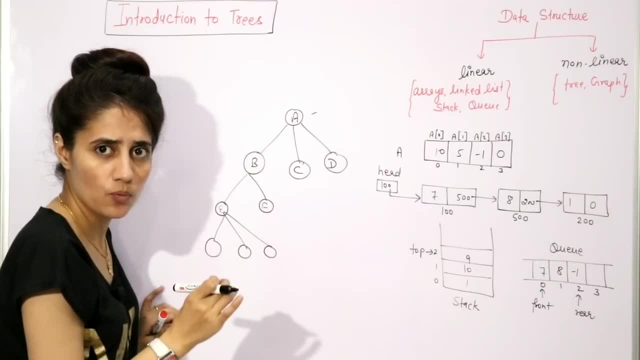 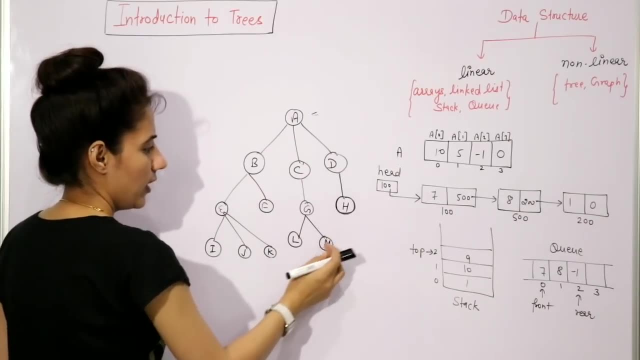 report to dean dean are going to report to the ceo. this is what a hierarchy. it's not like that faculty is directly going to report to the director of the college. so here i have added some more notes. so this is what a date these this is. 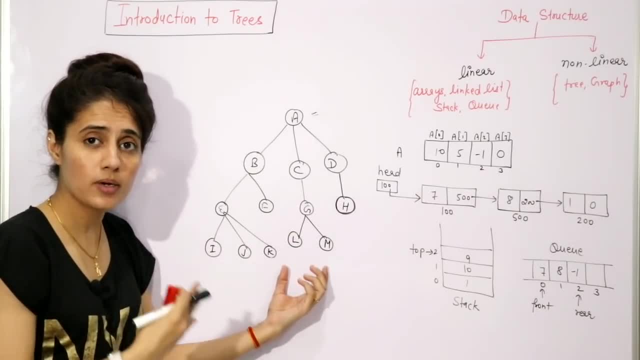 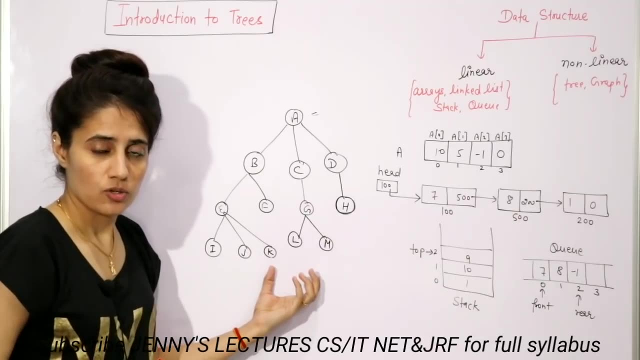 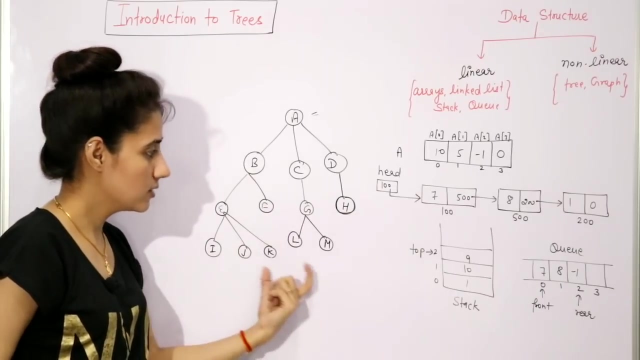 data items which are having hierarchical relationship among them, right? So you can say: tree is what? Tree is basically a known linear data structure which is going to simulate this hierarchy. Tree is basically going to represent this hierarchy. or you can say: tree is used to. 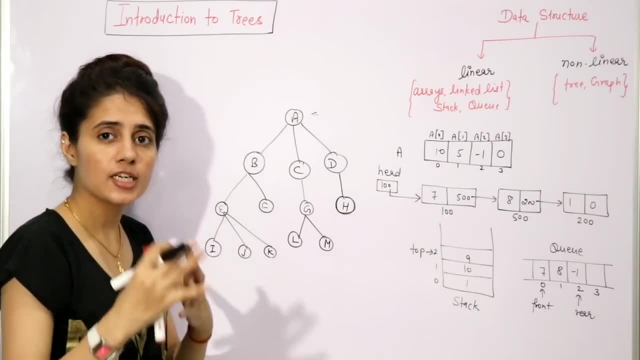 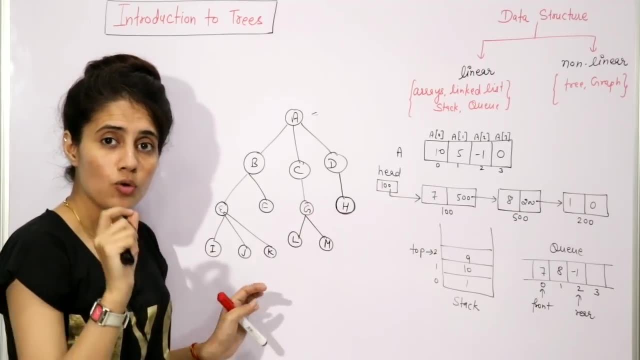 represent the data items which are having hierarchical relationship between them. So now, this is what the logical representation of tree in data structure See. you have to figure it out in which context you are discussing the tree Tree in the context of graph theory. 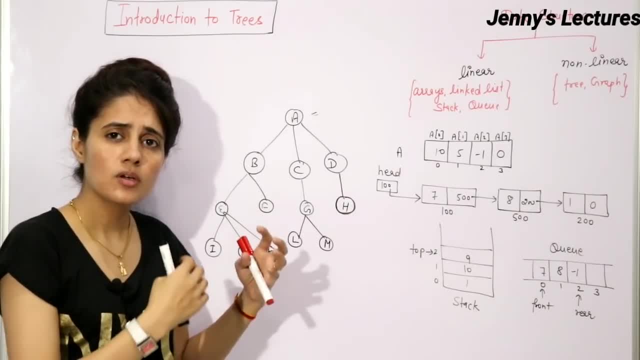 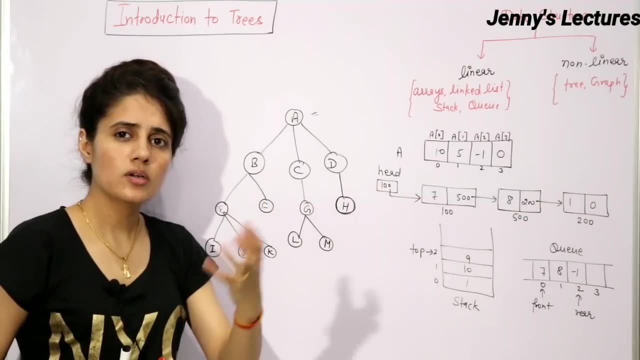 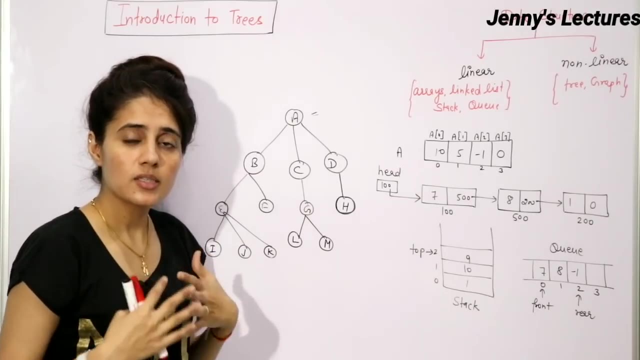 or in the mathematical form, or tree in the context of computer programming or data structure, because in that case, in the graph theory we are considering, that tree is what It is: an undirected graph which is connected and acyclic, right. But here, when we are discussing the tree, 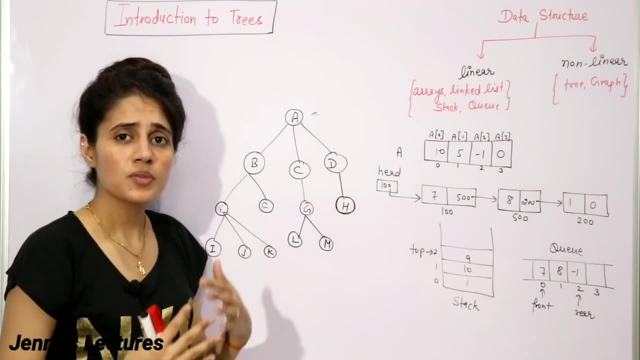 in the form of in the context of data structure, we are considering that tree is what It is: an undirected graph which is connected and acyclic, right. But here, when we are discussing the tree in context of data structure, here we consider that tree. this is having a direction. See here, if 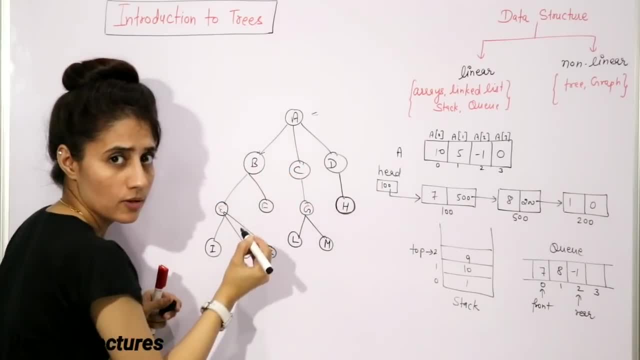 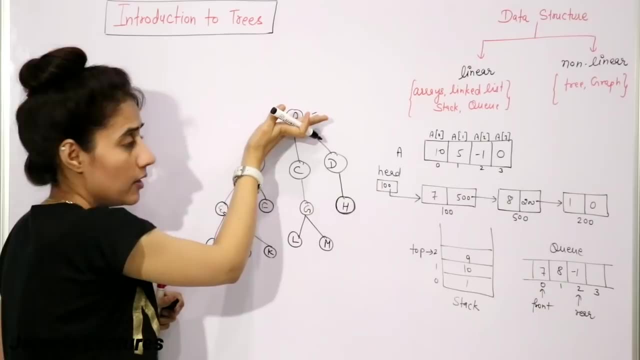 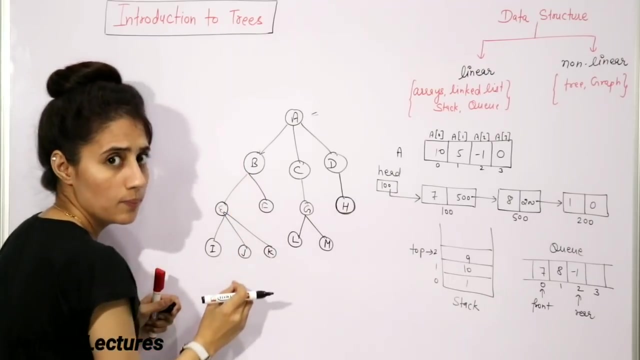 this is a tree. in that case you can go from A to B, but you cannot go from B to A. So tree basically grows from here top to bottom. We can go from B to E F. you cannot go from E to B. 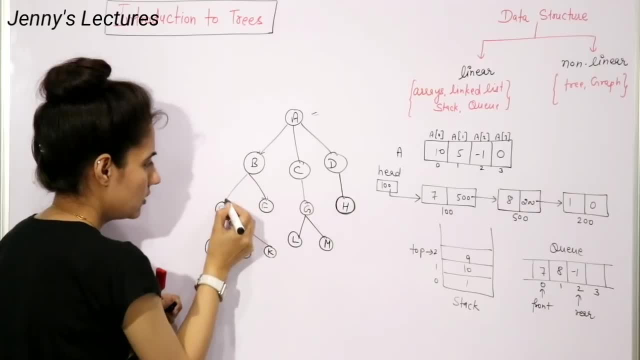 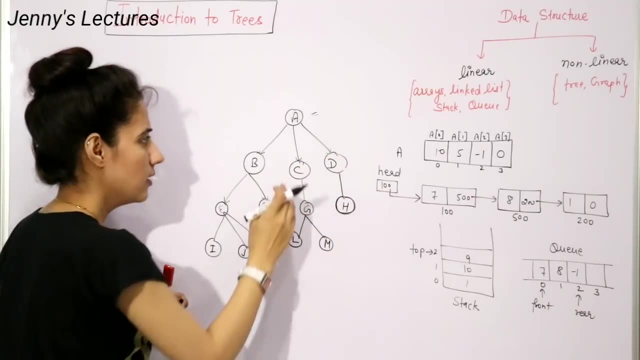 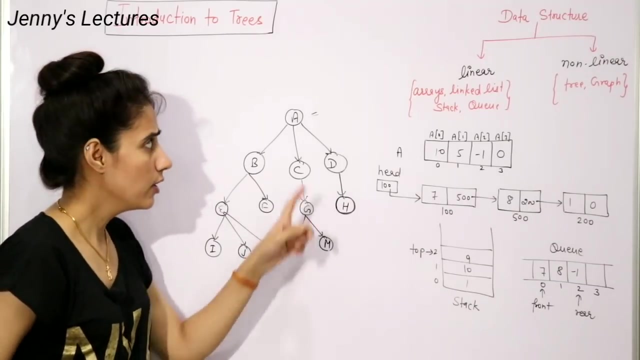 sorry, sorry, F to B. So this is, you can say a direction, Right, Somewhere it is represented with directions and somewhere it is represented without directions. But if you represent it without direction, then also the rule is what, The condition is what You can go from top to bottom. You can go from A to B, A to C, A to D. 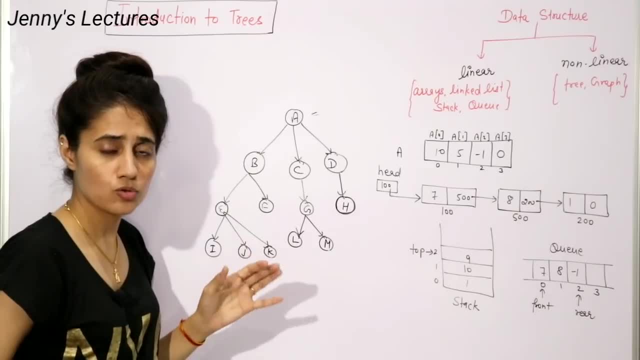 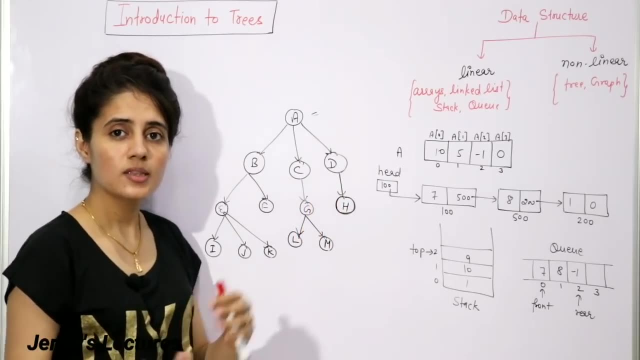 but you cannot go from C to A. This is the case. So by default it means the direction is from here to here, from top to bottom. And if you compare this tree with the actual tree, then there you can say that tree basically grows from here to here, from top to bottom. So this is. 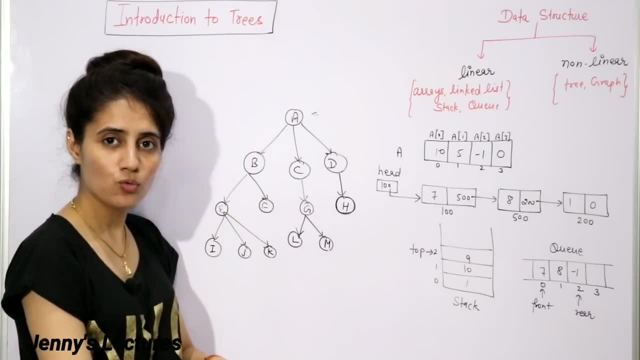 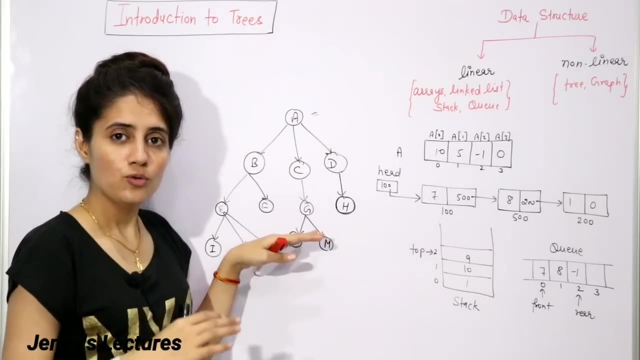 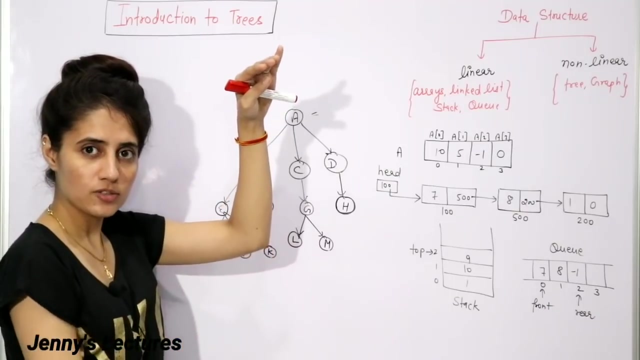 that ground into the air. We have roots, we have branches, we have leaves, Right, But this basically grows from top to bottom. So when you you can say, flip that actual tree upside down, then here you will have roots. then you can say: we have branches and leaves, So here in this tree, 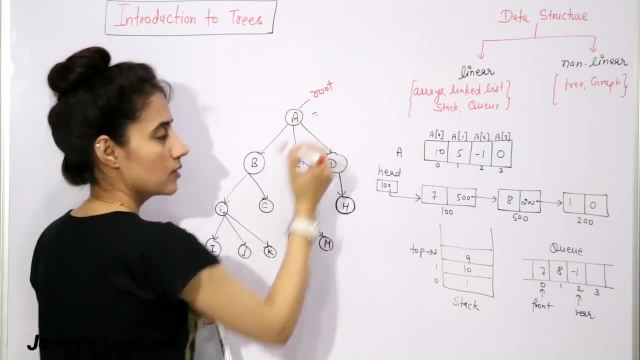 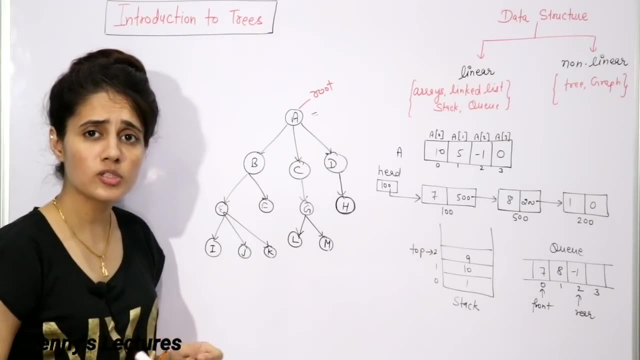 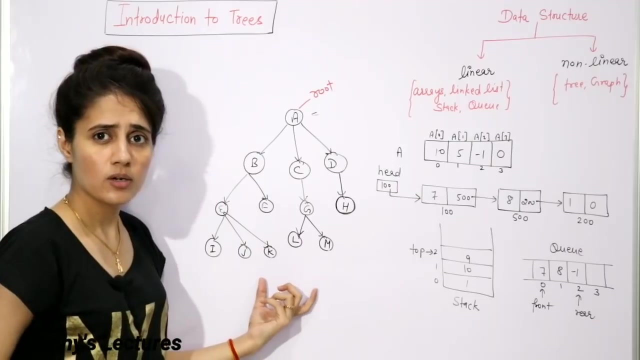 also this is known as what Root Right And these are known as nodes Right Nodes means they are going to store some information. So this is going to store some information here that here I'm, you know, represented this tree of that college hierarchy, So it is having person name or 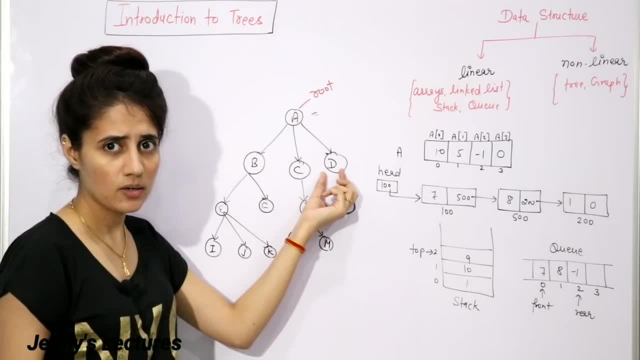 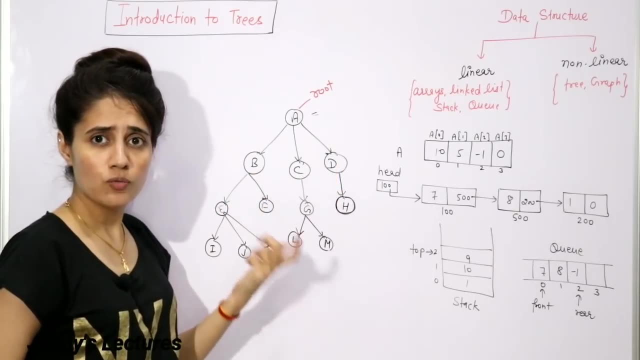 something like this: or person name and designation of that person, Right? But here I'm just writing A, B, C, D, Right? So the tree, the nodes, can have numbers also: 1, 2,, 3,, 4.. The nodes can: 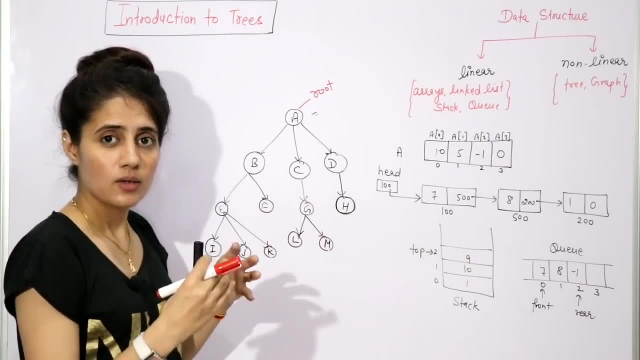 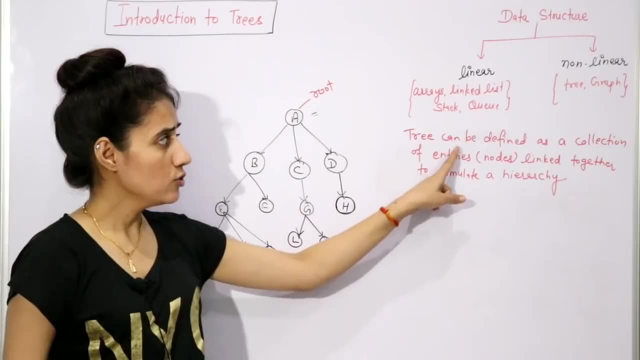 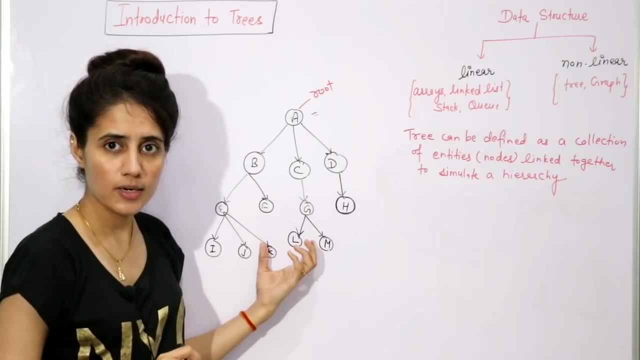 have characters also, The nodes can have strings also, But the main thing is what Nodes are having some information. So how can you define a tree? See, tree is what It can be defined as a collection of elements, or here we call not elements, here we will call nodes. Right In array we call elements. 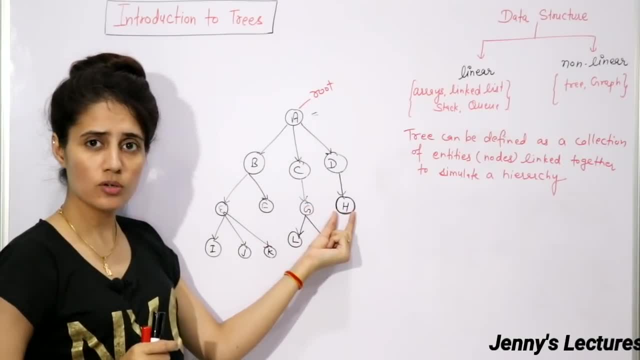 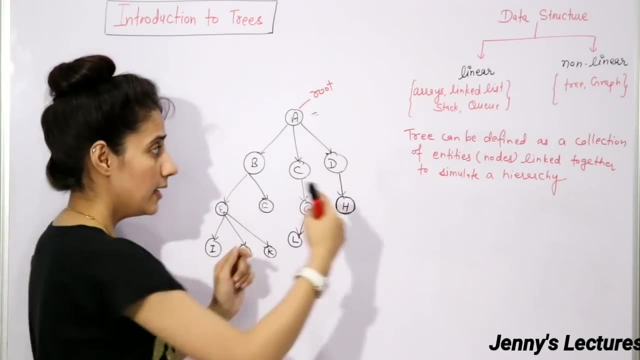 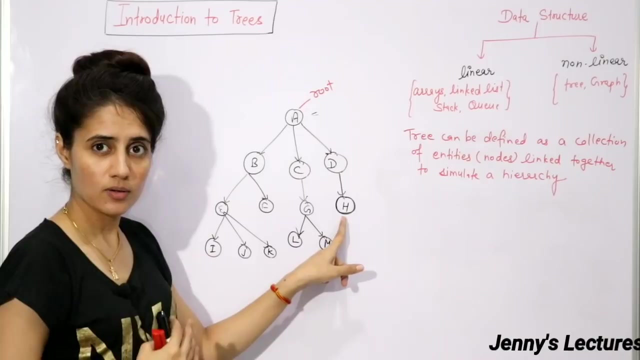 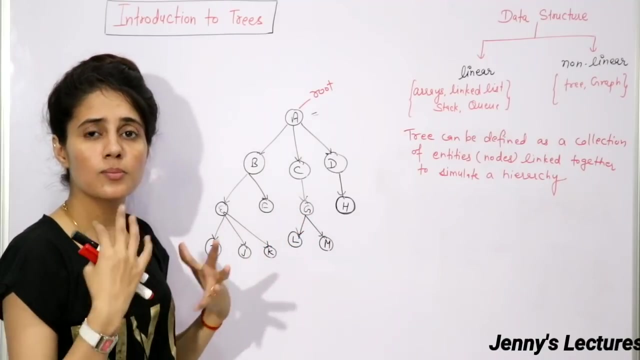 In linked list, we are calling nodes, and here also this, this is what known as node, Because this is containing information as well as link to the next one, Link to its. you can say it is what Successor of this node, Right, So this is what a node, So it is what a collection of nodes which are linked together to. 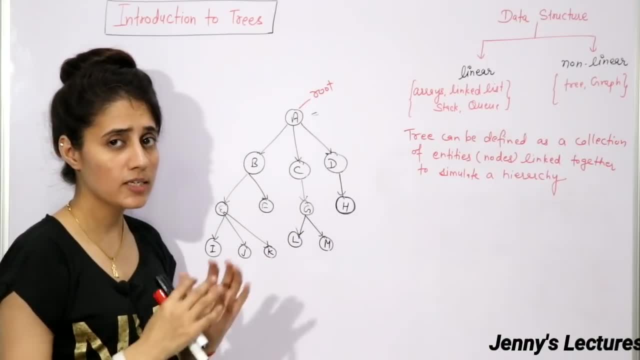 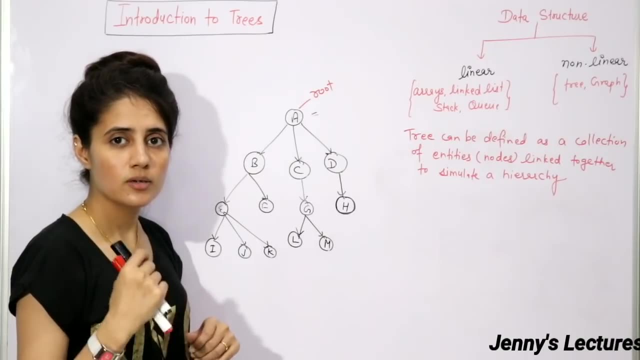 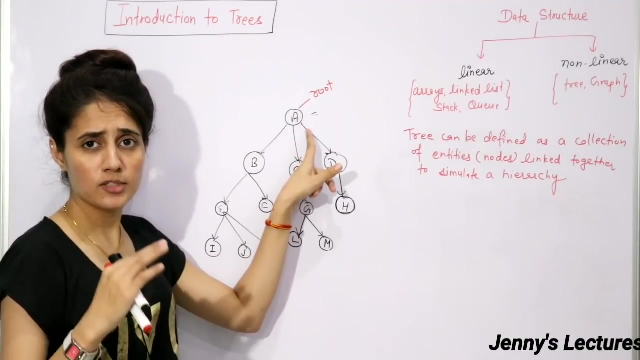 simulate a hierarchy. This is what a tree. It is a non-linear data structure. Fine, Now we will discuss some basic terminologies used in tree. Fine, First, is what Root of a tree? Root means the topmost element, Right. Or you can say root, this is not having any parent, The node which 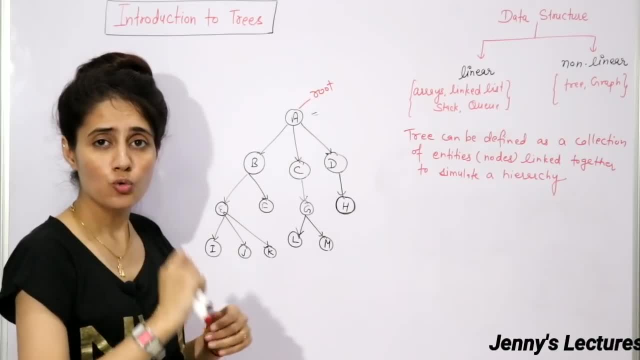 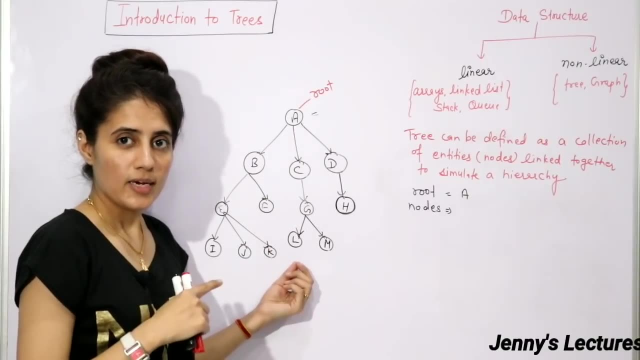 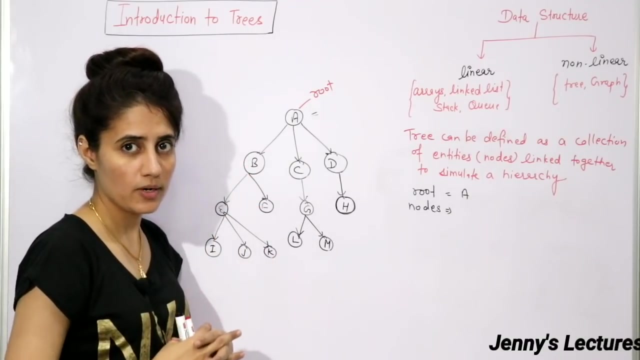 is not having any parent. that is known as root node of the tree, The topmost element or the first element in the hierarchy that is known as root. So here in this tree, root is what A Nodes Node is basically what, Which is going to store some information Right And also containing link to 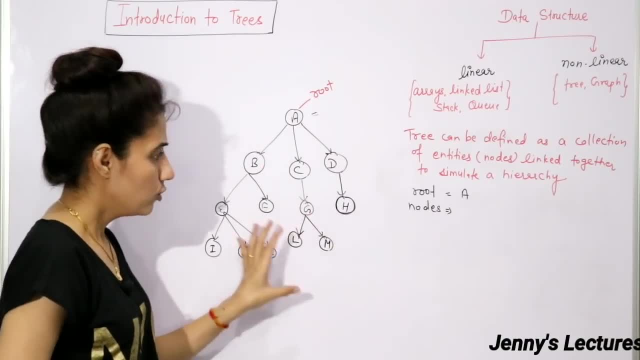 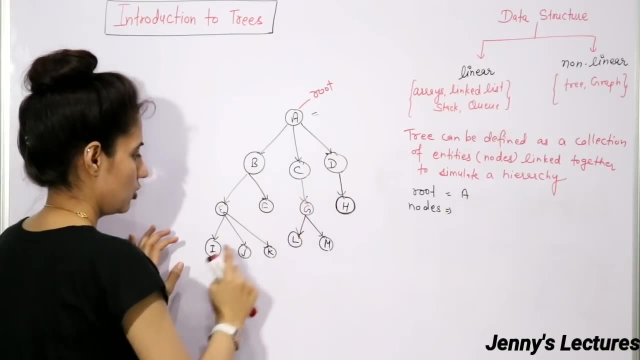 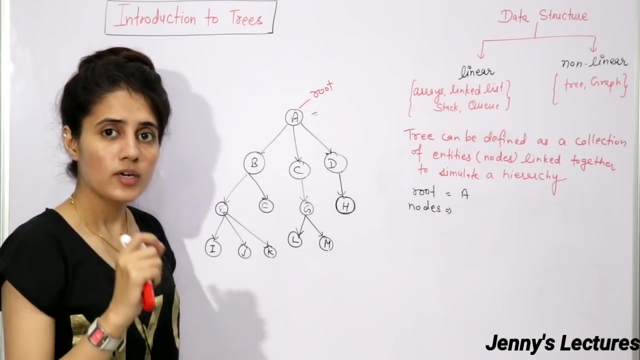 the another node Right. So now, here you can say this: elements of this tree are known as nodes. Elements from this tree are A, B, C, D, E, F, G, H, I, J, K, L, M. These are what Nodes of this tree. Fine. Next thing is what? What is a? 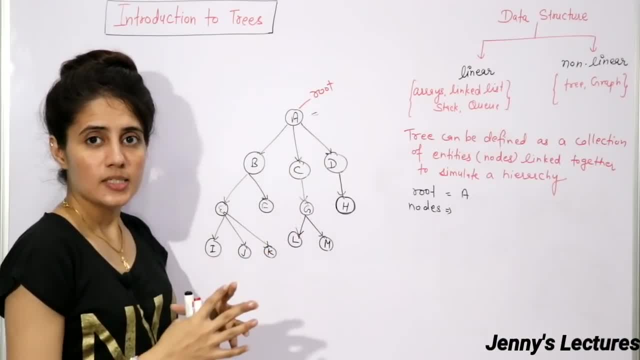 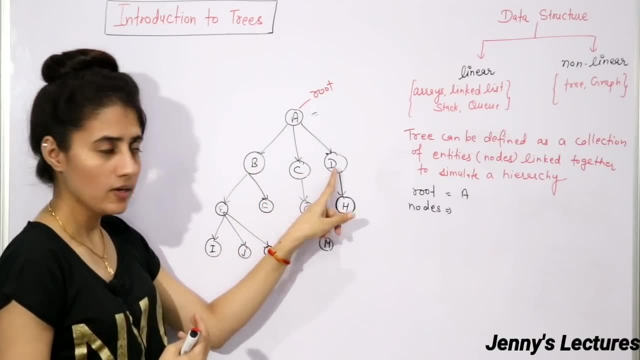 parent node. So here, I guess by looking at this tree you can easily say which is now parent. In this case, See A is parent of B, C and D, Fine And C is what Parent of G. So parent definition. 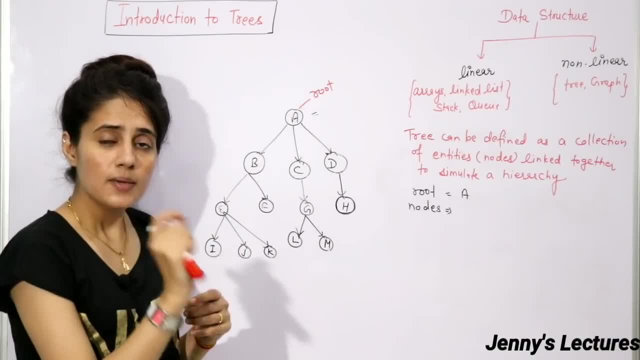 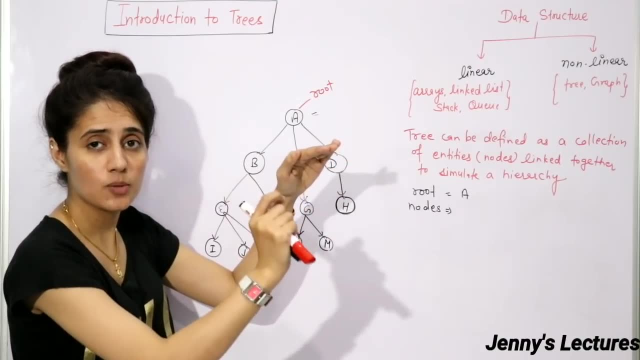 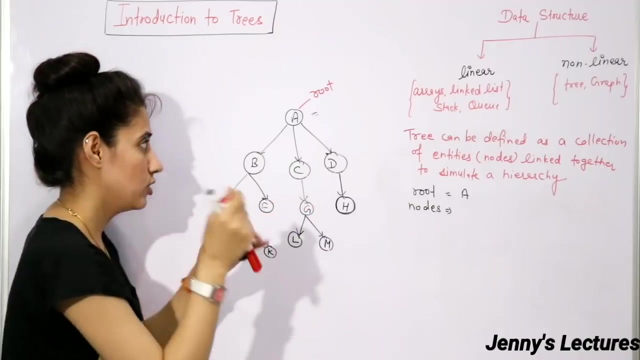 what you will see: Parent node. The definition of parent node is what The immediate predecessor of any node is known as parent of that node: See immediate predecessor. Predecessor means previous node to that node And second term is immediate, Immediate predecessor. 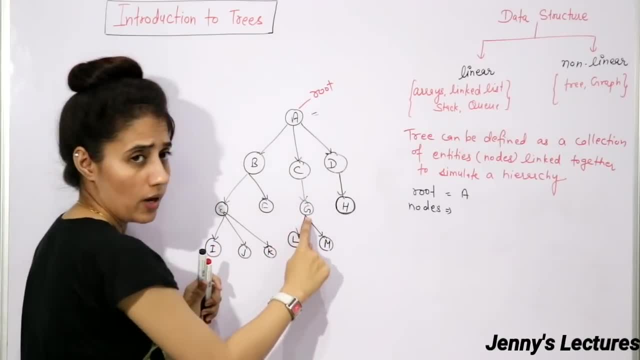 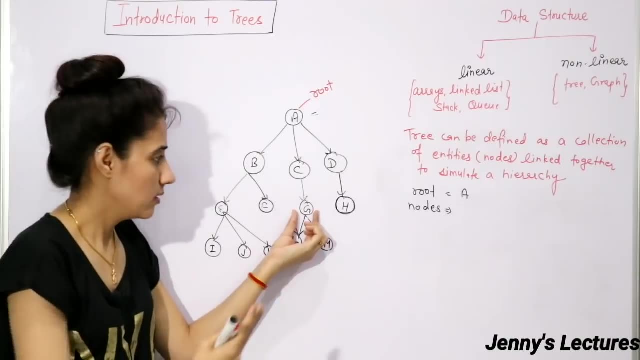 See, you can take any node. I am taking G. Find out the parent node of this one. So find out the immediate predecessor. Immediate predecessor is C. So this is what Parent of G. Now what about A? 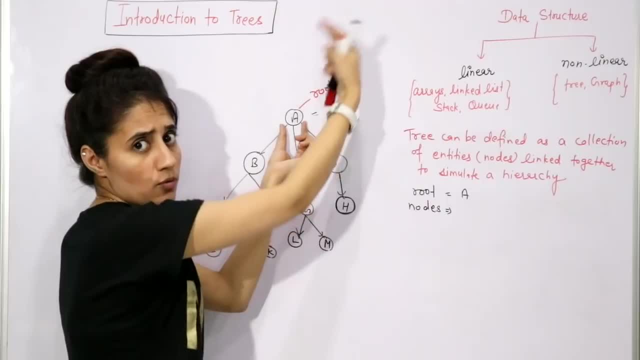 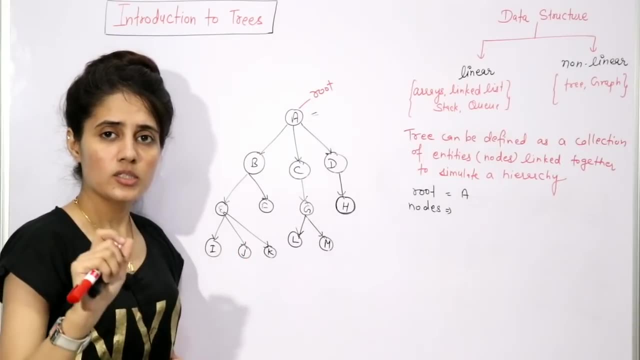 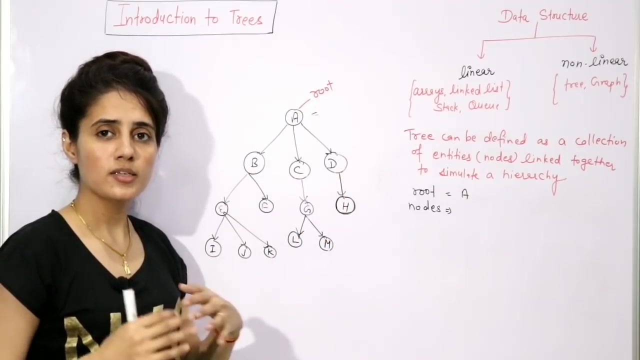 Is there any immediate predecessor of this node? Previous node: No, This is the first node only. So root is not having any parent node. Now, what is child node? So child, you can say the immediate successor of a node, is known as child of that node. See Now, what about A? If you say: 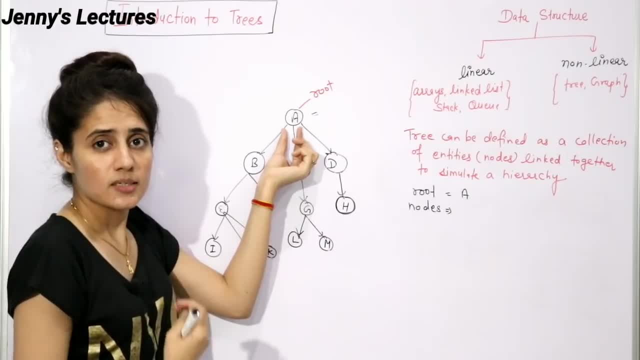 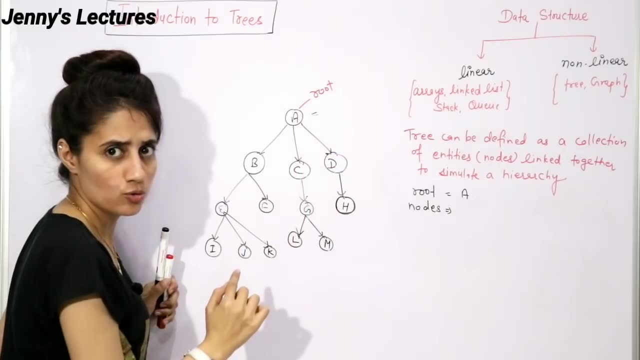 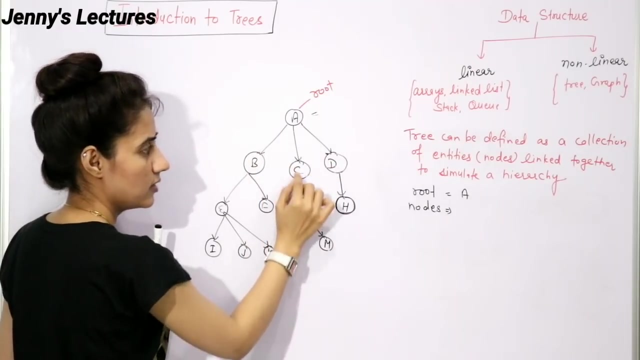 what is the child of A? So the immediate successor Successor means the next nodes, Immediate successor of A. So the immediate successor of B is the immediate successor of A. Okay, Okay, So in this case the immediate successor is B. Let's go to the next node. will say A. 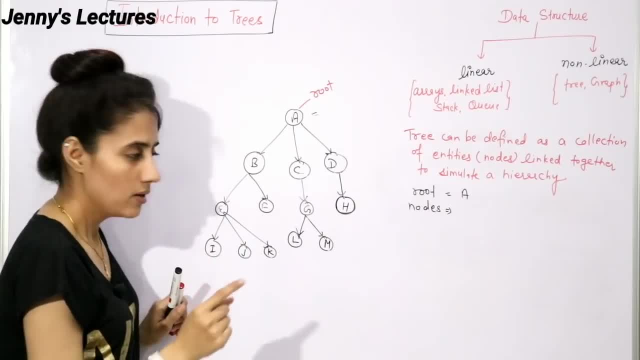 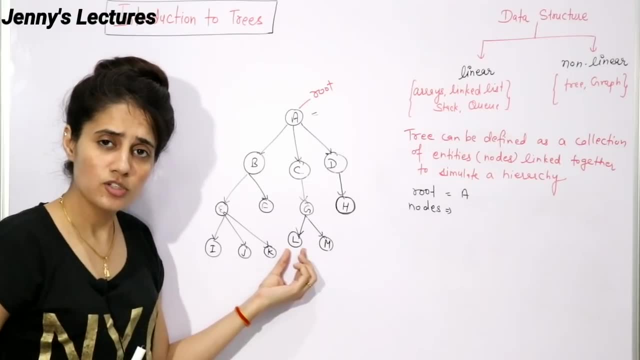 Actually the immediate successors are children of a. that one, two, two, even though the immediate successor are children of b, not the immediate separate successor. Get it So: intermediate successor of A. this is the immediate successor of A And then the秒 Hani-alth, who are one, two. 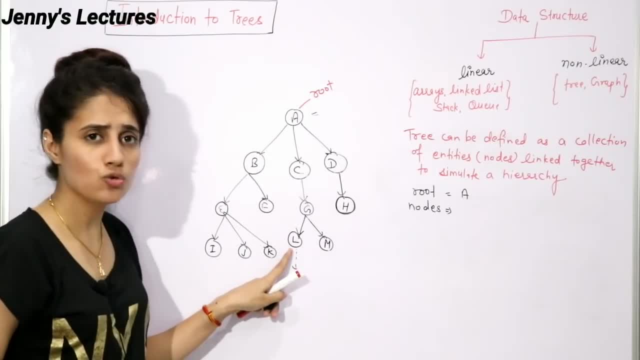 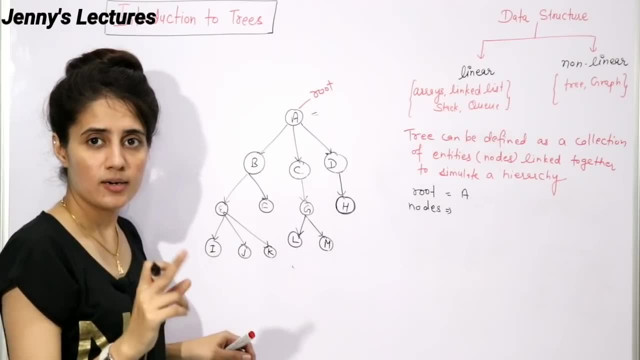 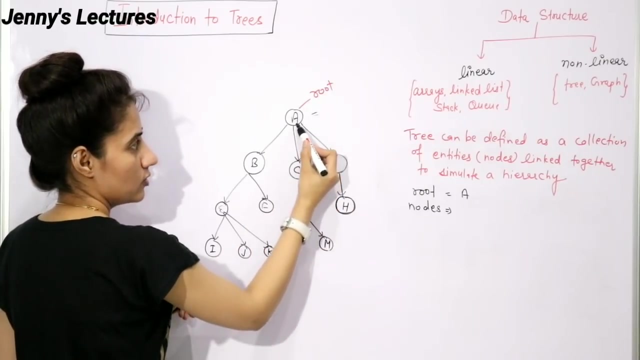 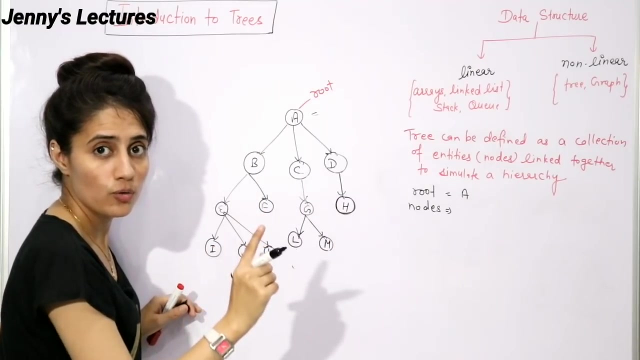 to L. No, we don't have. It means L is not having any child, Right. So these are containing what Parent, child relationship, Also grand parent also. See here you can say this: C is what Child of A, but C is what Parent of G. So what you can say This: A is what Grand. 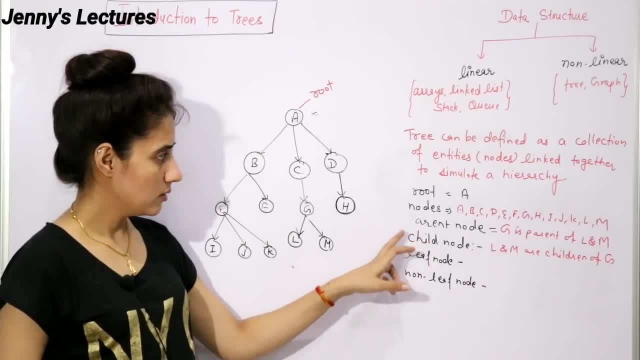 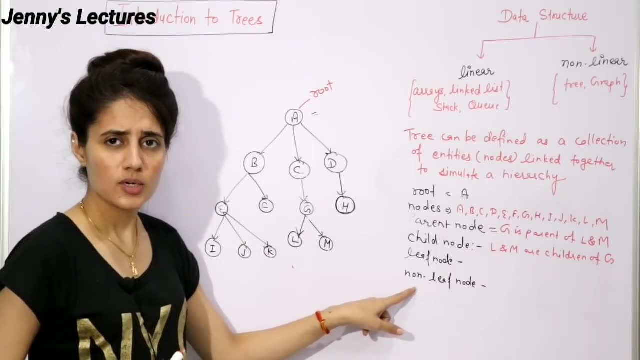 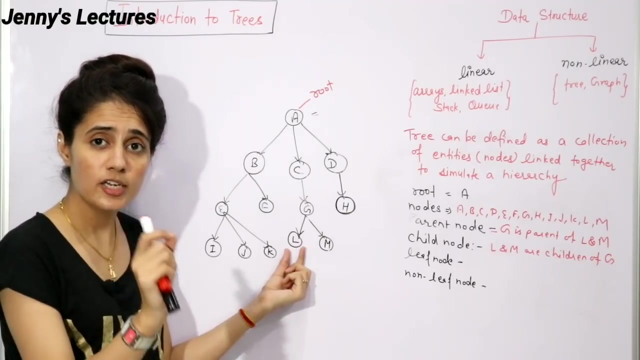 parent of G. So here I have written nodes. example of a parent node also, child node also. Right Now we will discuss what is leaf node and non leaf node. See this L. I have told you this L is not having any child. So the leaf node is what The node which is having? 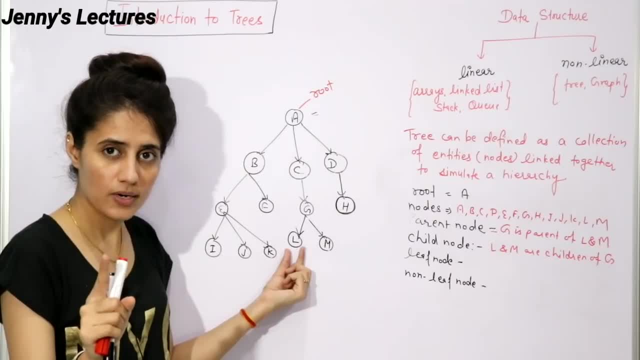 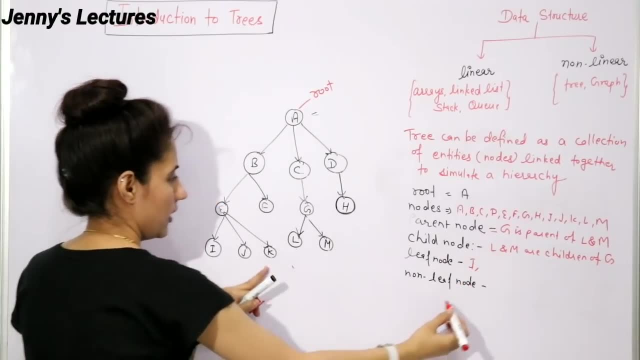 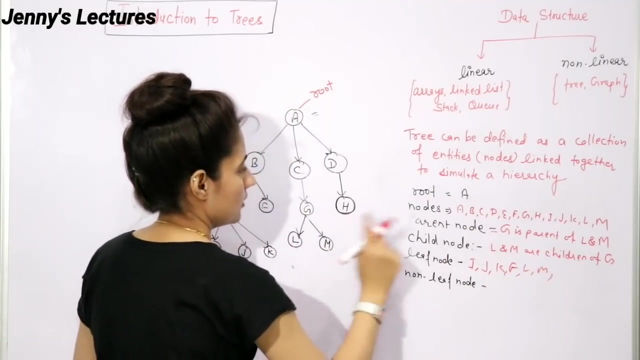 no child. That is known as leaf node Right. So here in this case, leaf nodes are C- I is a leaf node J and K and F is also leaf node. L and M are also leaf node, plus H. These are leaf nodes. 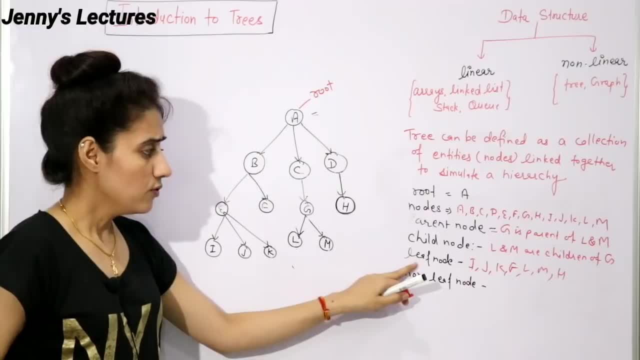 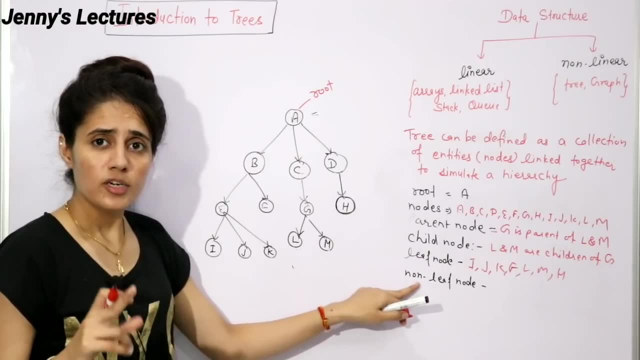 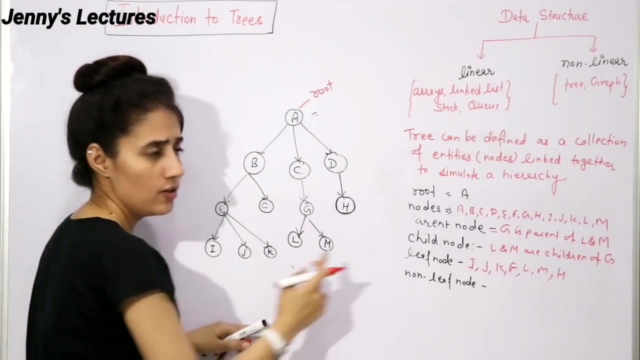 which are not having any child Plus leaf node, are also known as external nodes. You have to take care of this thing. External nodes, Right. So now what is non leaf node, which is having at least one child, Right? So all the other node except leaf nodes are 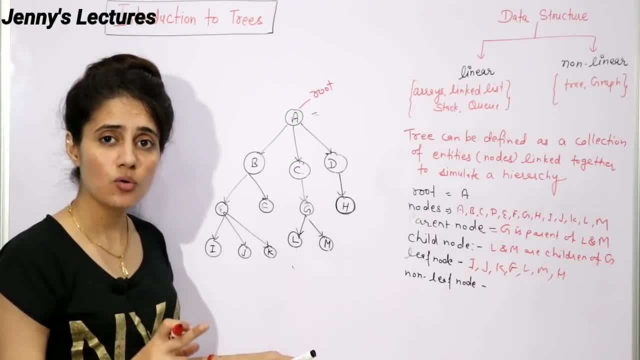 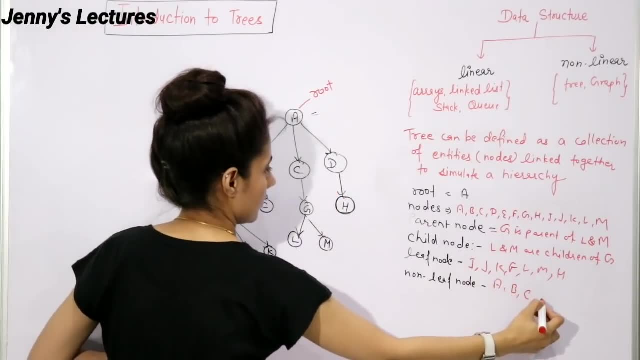 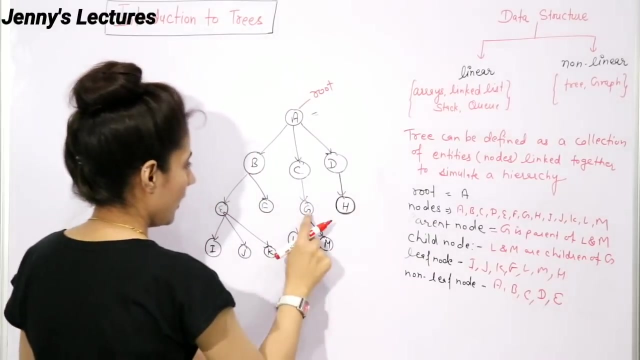 known as non leaf node. So what is non leaf node? It is having at least one child, Right? So these are known as non leaf node As well as these are known as internal nodes. So here non leaf node are A, B, C and D also, plus E and G, Right, These are non leaf node. 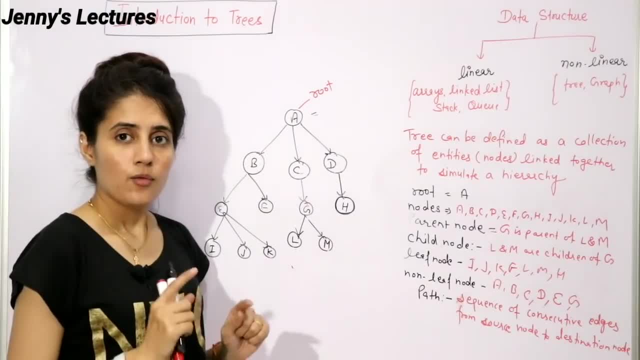 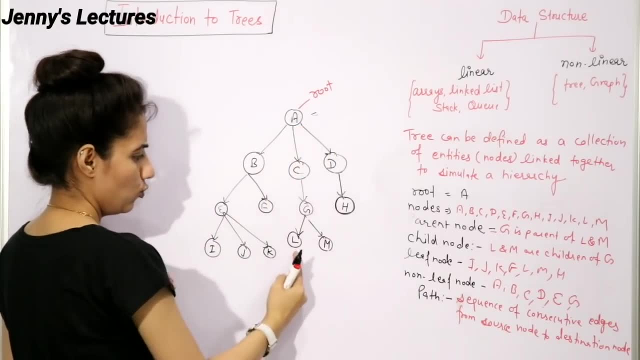 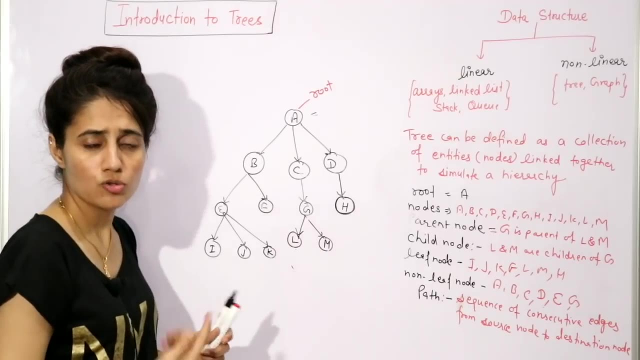 and you can say: these are internal nodes. Now, next is path C. If I ask you what is non leaf node, How you can go from A to L, Right, You will say from A to C, then C to G and G to L. So this is what, This is, what a path Right? First of all, this edge, this edge and this. 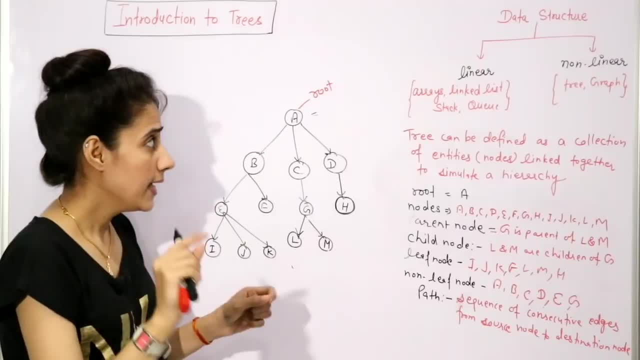 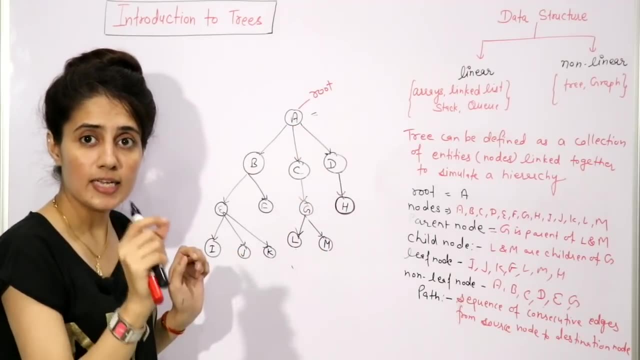 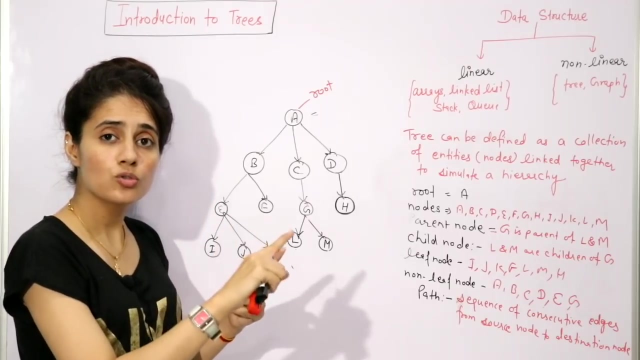 edge. Right See, edge is what Link between two nodes? These are nodes, and the link between A and C is what This one. So this is known as an edge. So path is what You can say. it is a sequence of consecutive edges from source node to destination node. If I am asking you, 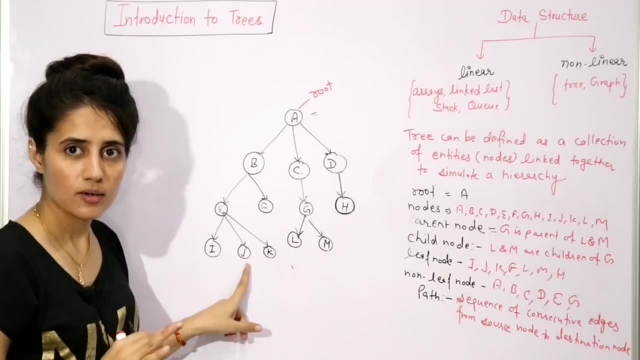 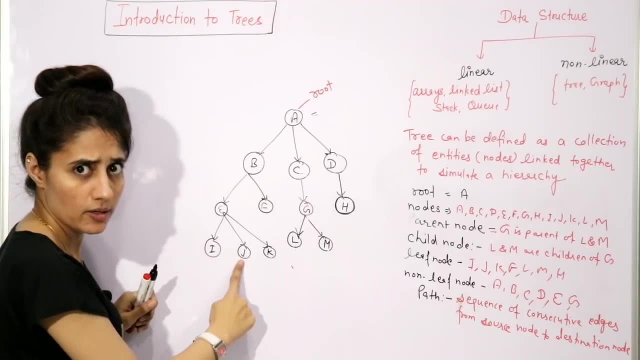 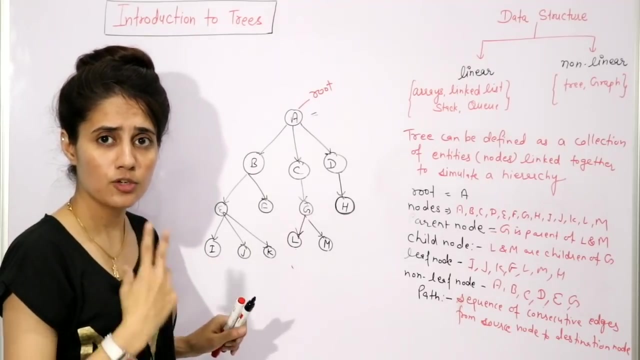 the path from B to J, then the path is what? From B, I will go to E, then from E to J. So path is what? B, E and E, J, These two edges. So this is what known as a path Sequence of consecutive edges from the source node to the destination node. Right Now, this is 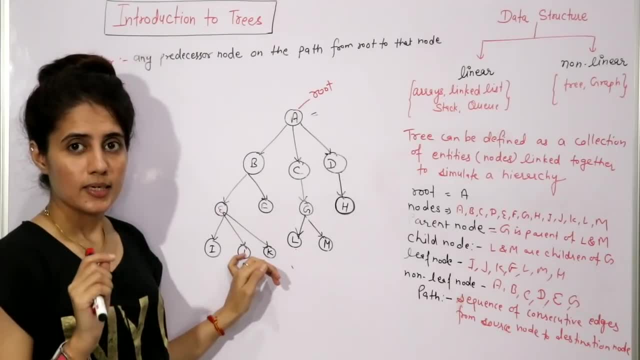 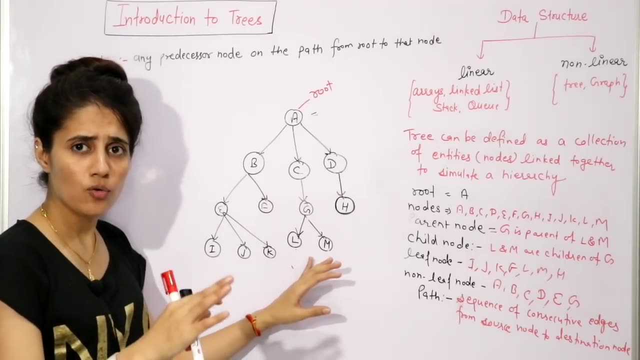 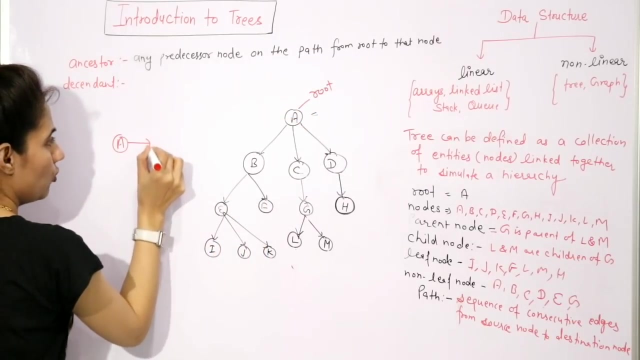 known asesenl values. anyways, We will see ancestors and descendants. See, ancestor is what Simply, in simple terms, you can say here in this tree, if you can go from a node A to B. it means: see, like this one, If you can go from this A node to B, node Right And see. 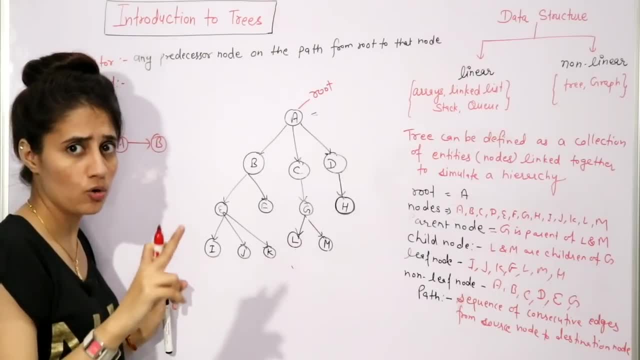 one more thing you need to take care: These links are unidirectional, not bidirectional. I have told you earlier also Right, So now here: a is what Ancestor and descendants. So this is what it means: you can sort them. down and evaluate if one node is databases or use some other nodes. Right, We will see 4 ones here and be holding this here곤 Framework and so forth. So a path isn't some taking judgingacress and other nodes, So we will see ancestor and descendants things. So in an stop pnf like this, we want to go to an entities. 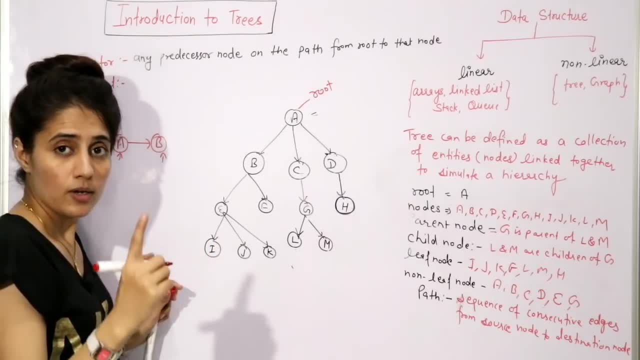 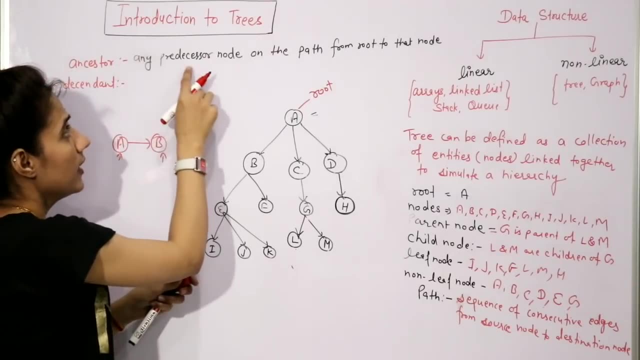 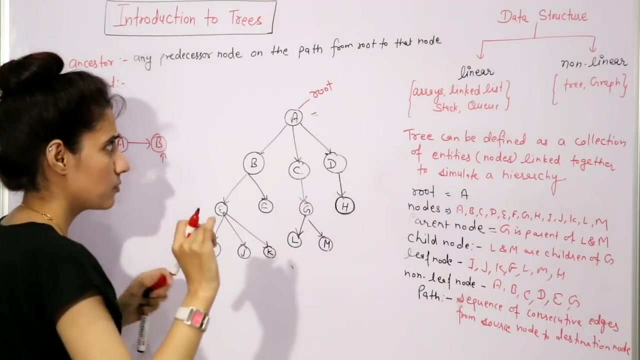 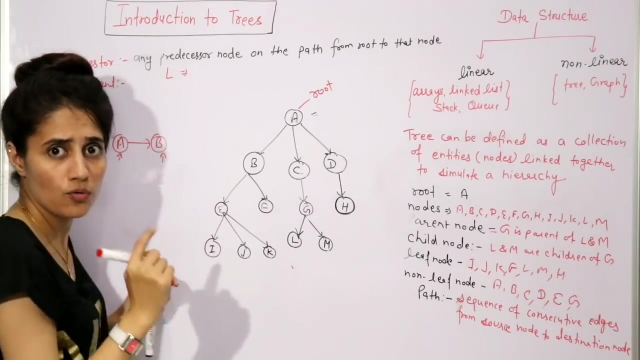 and b is what descendant? fine, and if you write, if you want to write down the formal definition, then you can say: ancestor of a node is any predecessor node on the path from root to that node. see now, if i ask you ancestor of l, then what you will say? ancestor of l? first of all, check out. 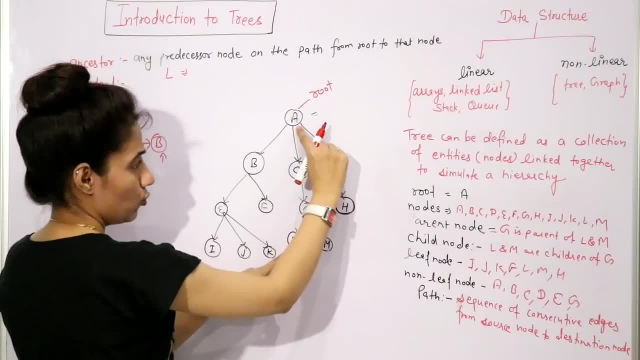 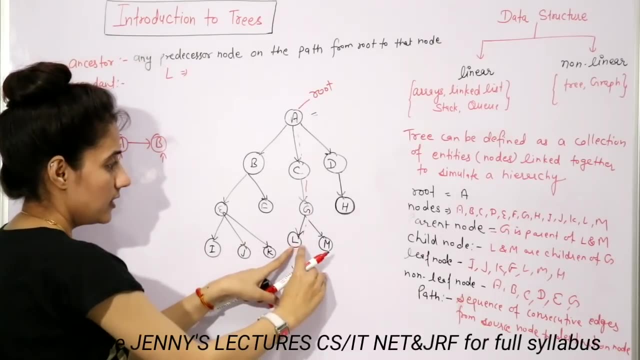 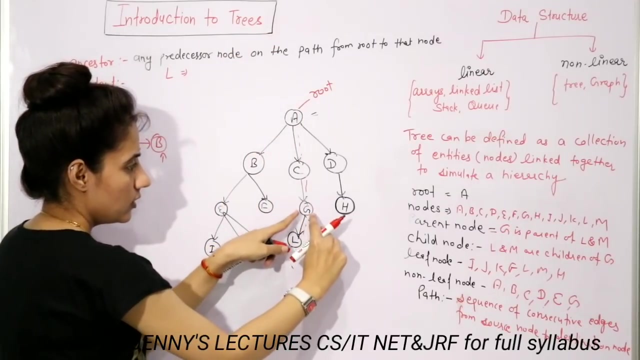 the path from root to that node, so from root. root is a root to l. the path is this one, this, this and this one right. so ancestor is what any predecessor node. predecessor means the previous ones, so predecessor node of l is what g also, c also and a also the predecessor on this path only. 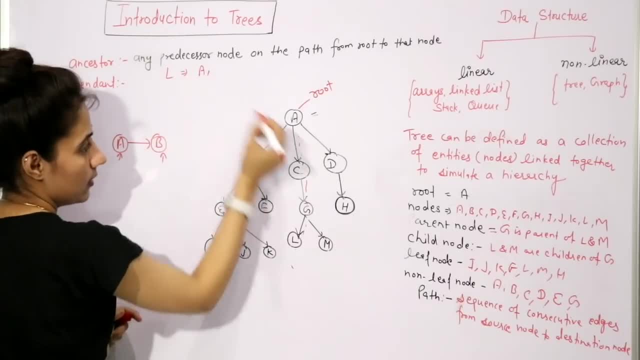 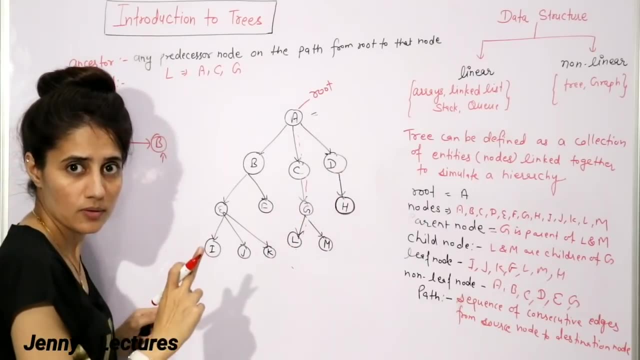 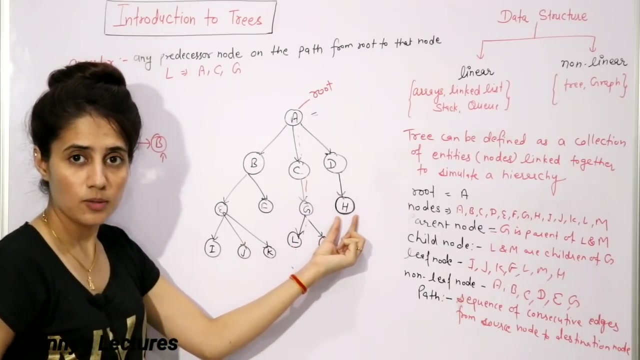 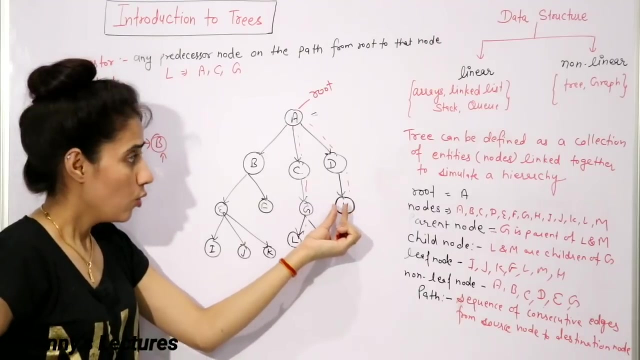 so ancestor of l is what? a, c and g, both, sorry, the three. you are ancestor of L right Now. if I ask you what is ancestor of H, it means find out the path from root to H, this one and this one. So ancestor of H is what? On this path, what are the predecessor? 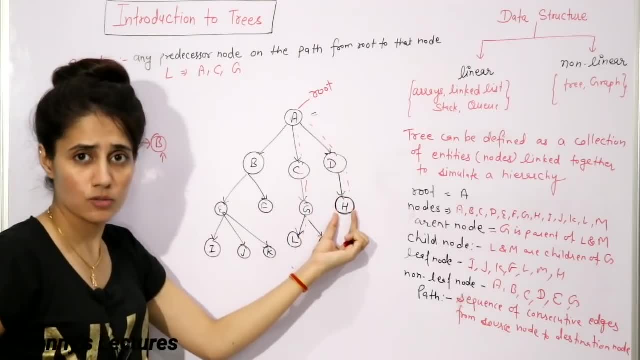 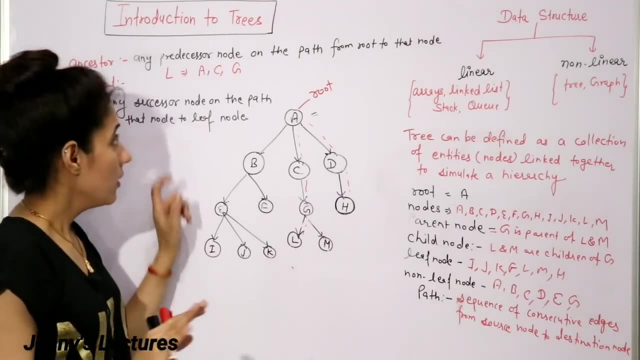 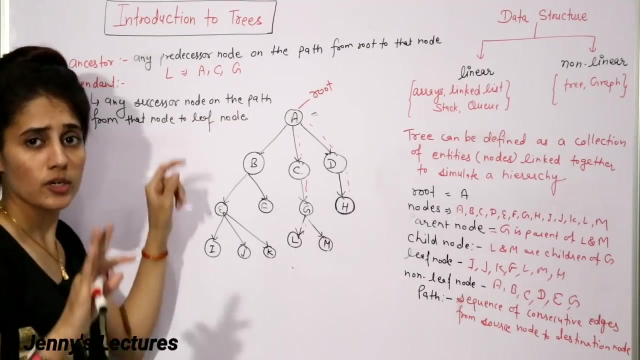 of H, D and A. So A and D are ancestor of H. fine, So now next is descendant. Descendant is what Any successor node on the path from the node, from that node to the leaf node See? 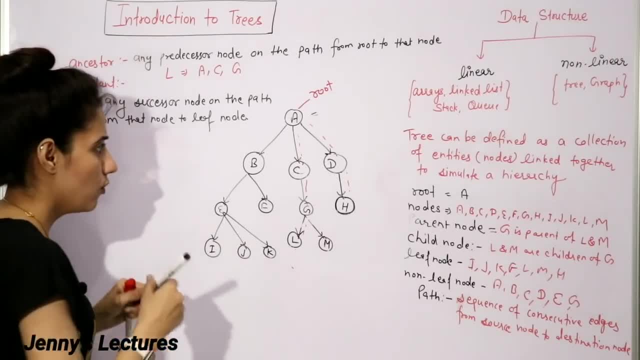 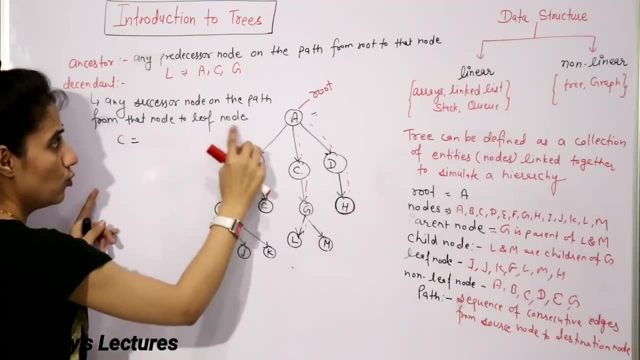 with example. if I ask you what is descendant of C, First of all find out the path. from that node means from C to leaf nodes. So from C, here I can go, I can go to G, after that I can go to L. 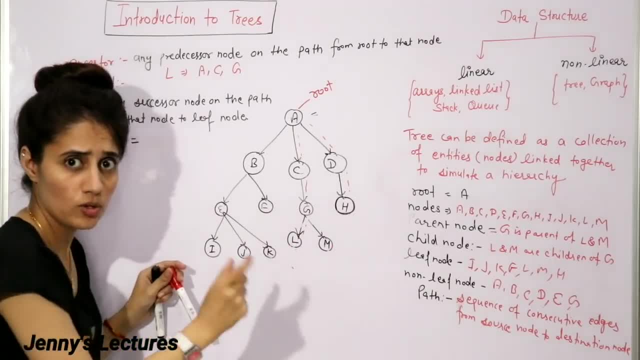 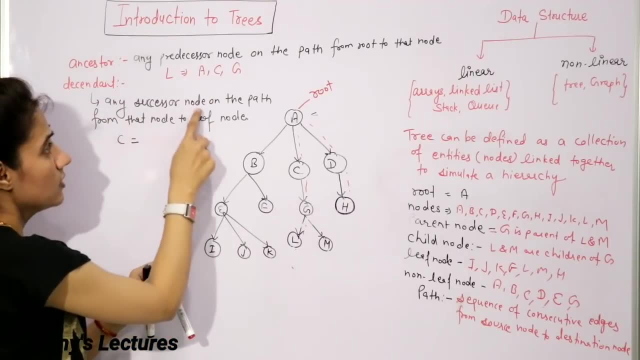 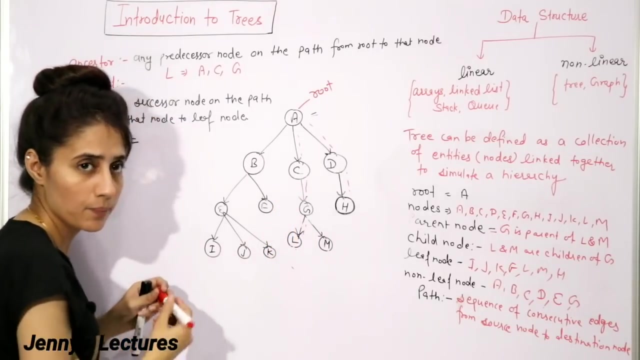 I can go to M also. These are leaf node. we have reached to the leaf node, fine. So these are two paths Means. so now any successor node. successor means after C, after C, on this path, successor node are G, L and M. So now here, G, L and M, all the three are what you 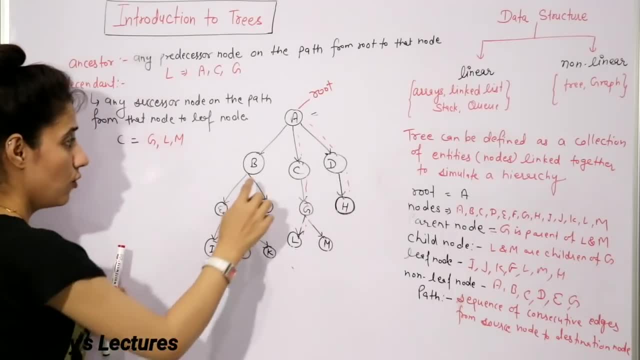 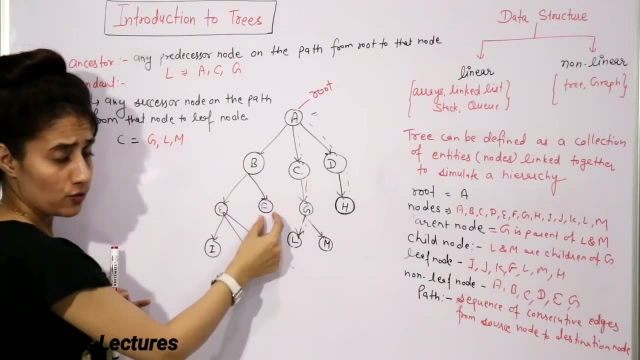 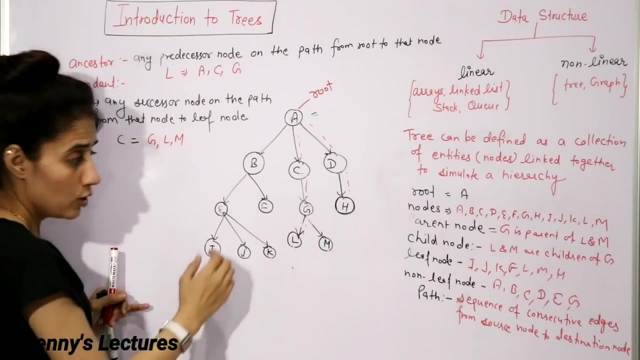 can say descendant of C. Now what is descendant of B? Right, find out the path from B to the leaf node. So F is also leaf node. So F is also descendant of B. Now, path is this one, this one, this one and this one, right? So 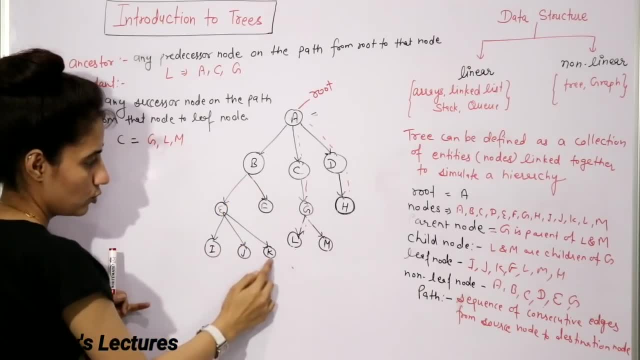 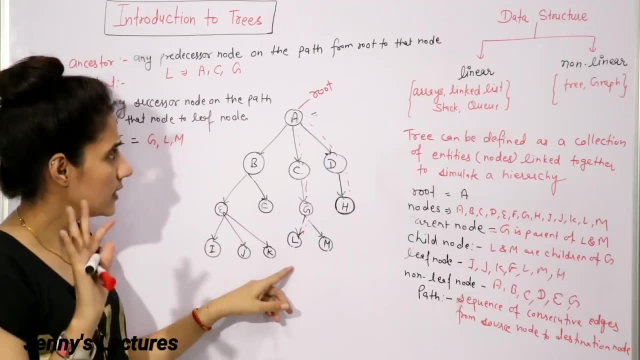 all these are descendant of B, E also, I also, G also, K also and F also. right, So these are descendant of B. See. now, if I ask you, what are the common ancestor of G and H? Ancestor means you. 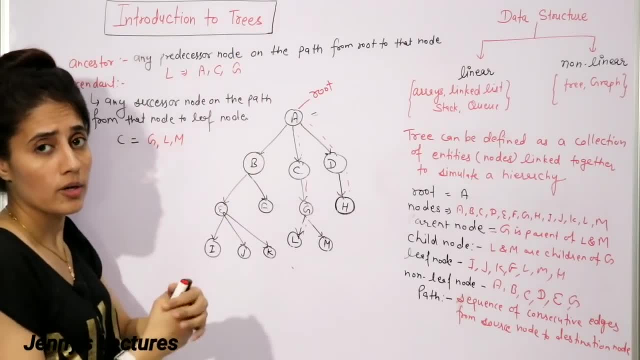 have to find out the predecessor node on the path from root to that node. Now, ancestor of G are what A and C, Ancestor of H is what A and C. So you have to find out the predecessor node on the. 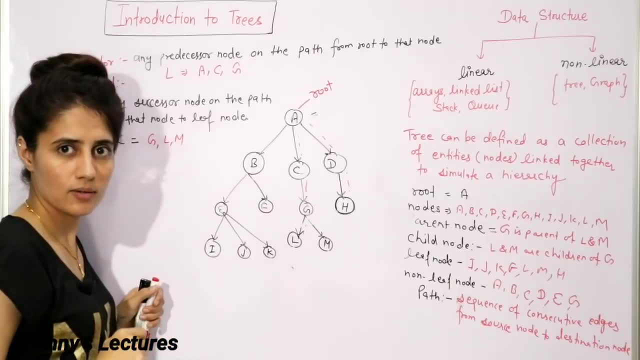 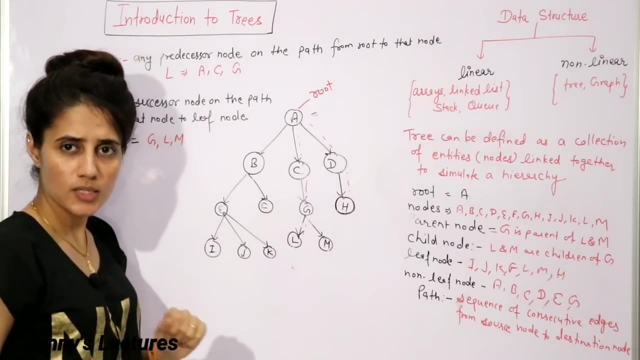 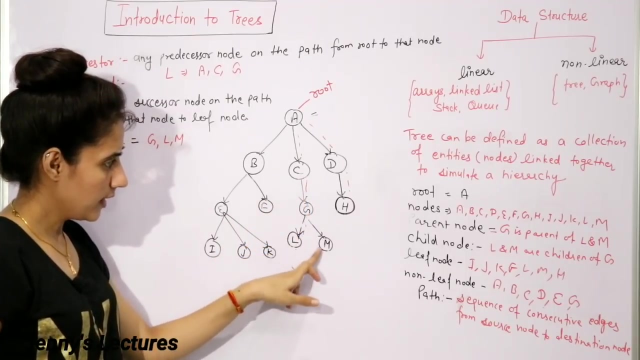 path from root to that node. Now if I ask you the common descendant of C and D, is there any common descendant? No, Why Find out the path from C to leaf node This one? G, L and M, these are: 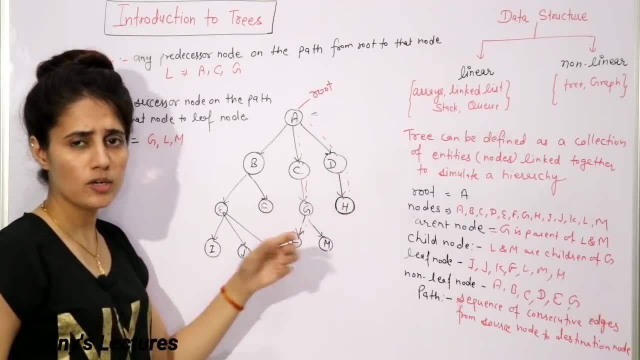 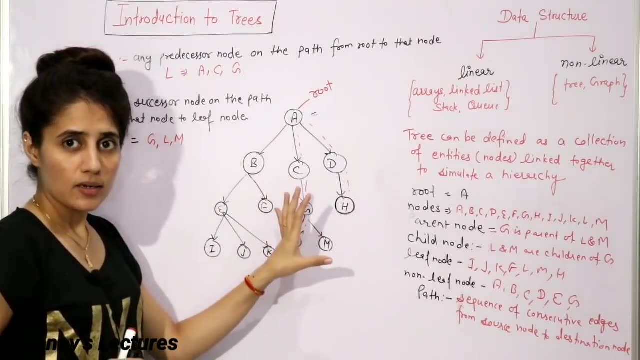 descendant of C. descendant of D is what H only, So there is no common descendant right Now. what is a subtree C? Suppose this is a tree T. Now the subtree of N is what A and D. So 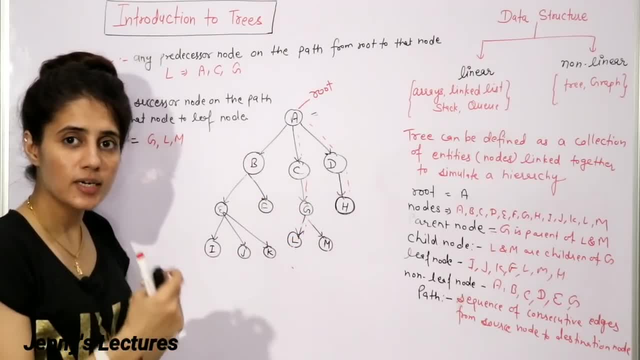 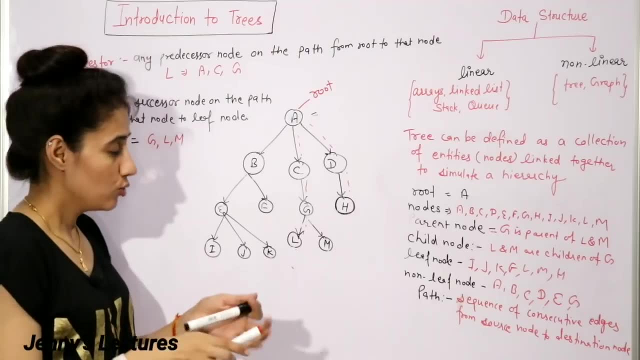 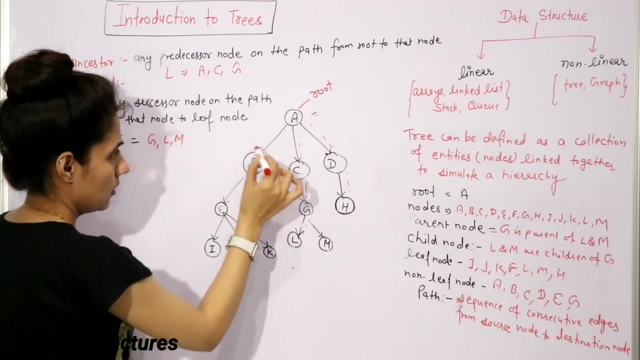 any tree, T is what You can say, which is containing a node of this tree T and all its descendants. right. So now, here you can say: the subtree is what Here, A is what The root, So the subtree of this is what, This is what A subtree, This is another subtree and this is 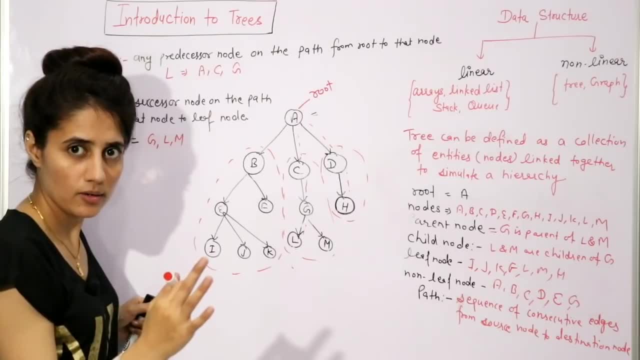 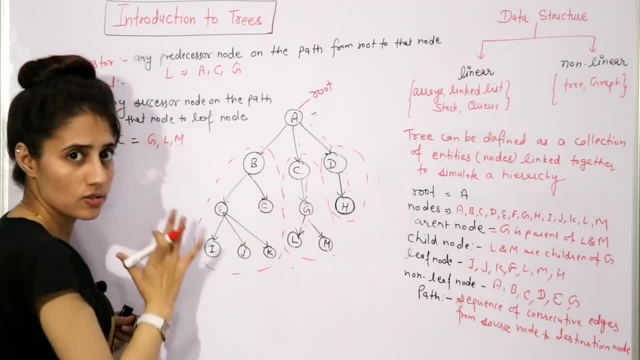 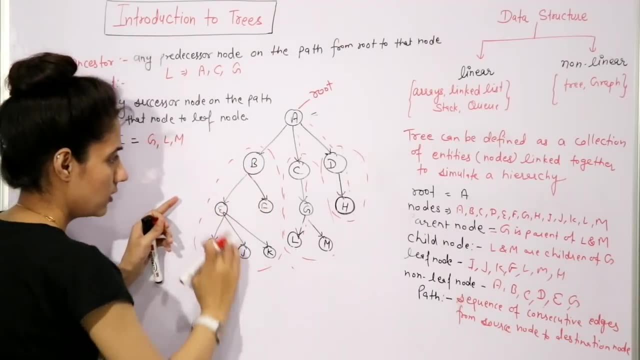 So this is what You can say. a node with all its descendants. So this is what One subtree, this is another subtree, this is another subtree Within this tree also, if you consider this one, so within this tree also, there is two subtree. One is this one, one is this one. 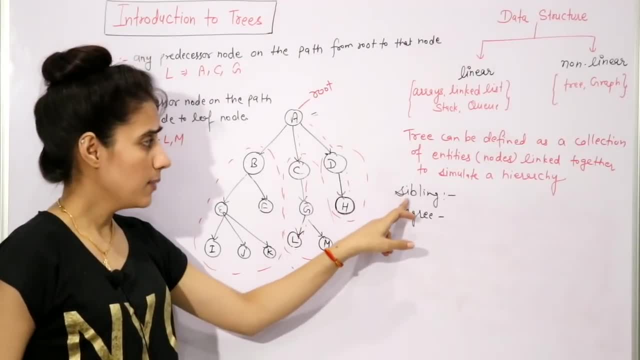 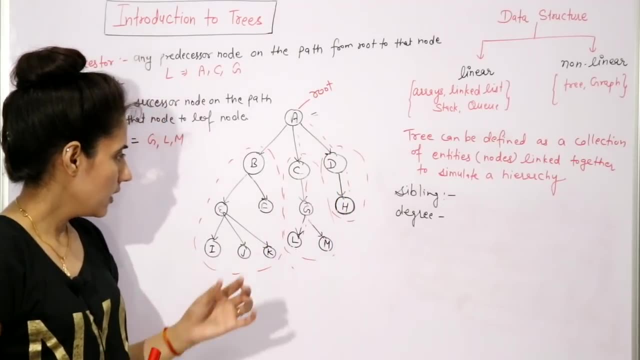 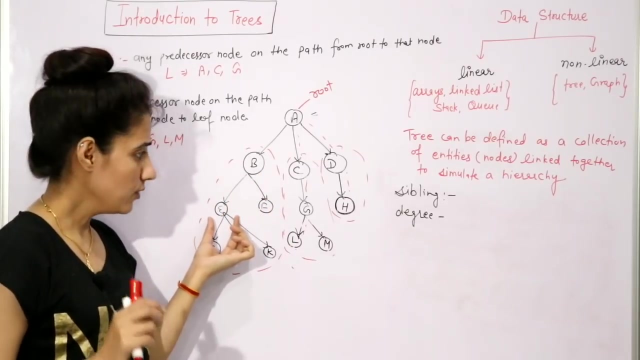 Now next is sibling and degree. Sibling is what All the children of same parent, Those are known as sibling. So you can say E and F. The parent of E and F is what Same, That is B. So E and F are sibling. Can we say F and G are sibling? No, See the parent of F. 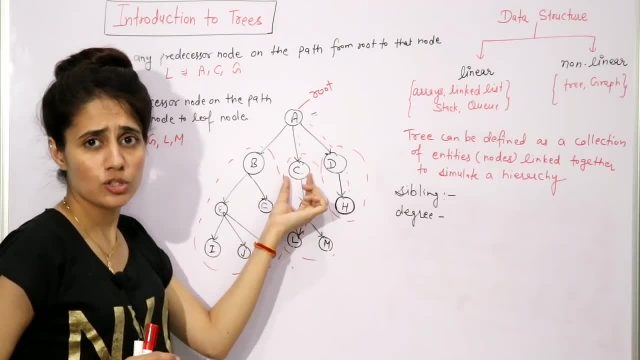 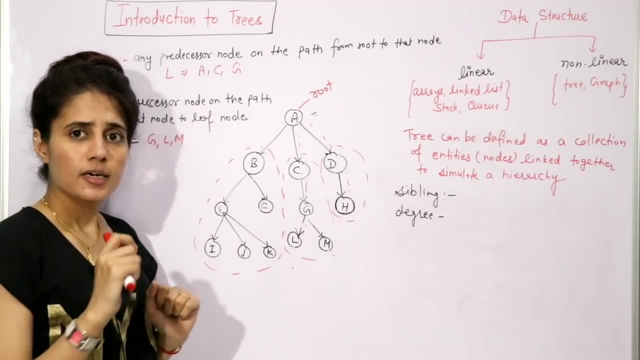 is what B, But the parent of G is what C Parent are not same, So these are not siblings. You can say: these are cousins. Fine. Now next is degree: Degree of a node. Degree of a node is what The 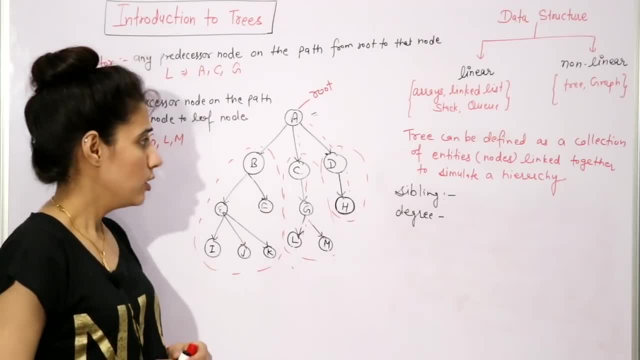 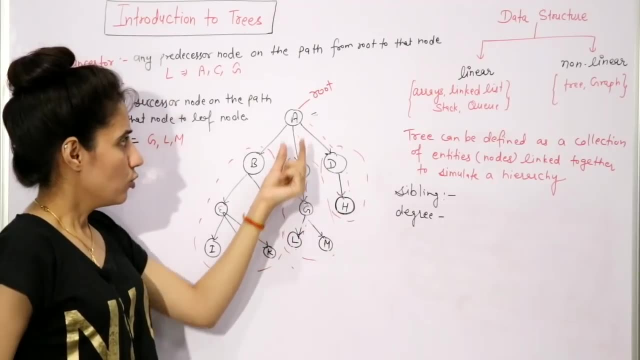 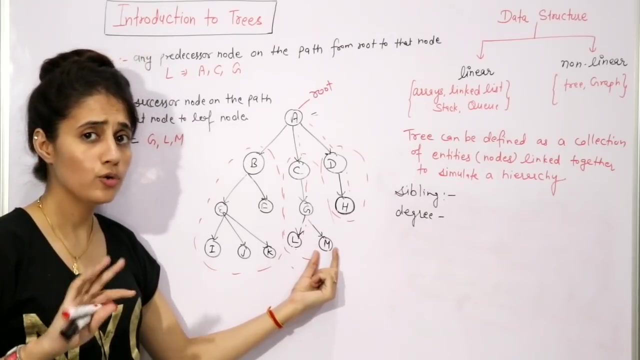 number of children of that node. Simple, That is degree of that node. So now if I ask you degree of A, you can find out easily: the children of A. So degree of A is what. 3. Degree of M: Is M having any child node? No. So degree of M is what. 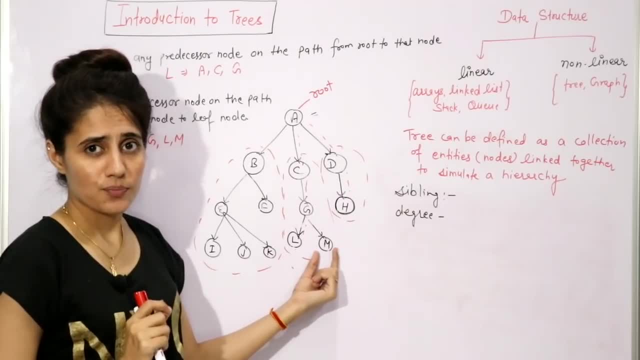 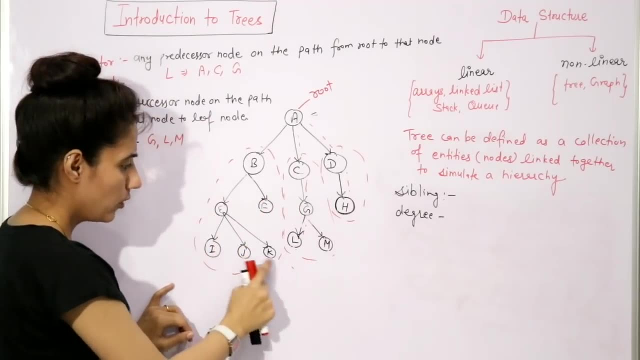 0. So degree of all the leaf nodes are 0.. Fine, Now see, degree of F is also 0. Now, degree of E is what? 1, 2 and 3. Number of children. Now, if I ask you degree of this tree, then what you can. 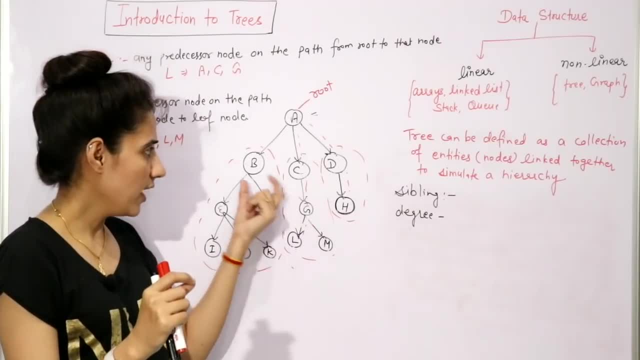 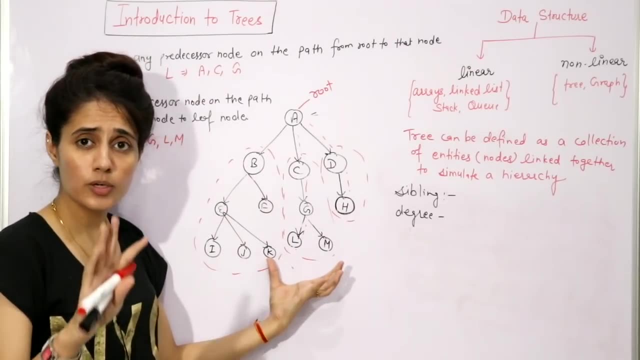 say The maximum degree of any node. So if I ask you degree of this tree, then what you can say, The maximum degree of any node. That is known as degree of this tree. So the maximum degree in this tree is what? 3 only Right, Because no node is having more than 3 children. So the maximum 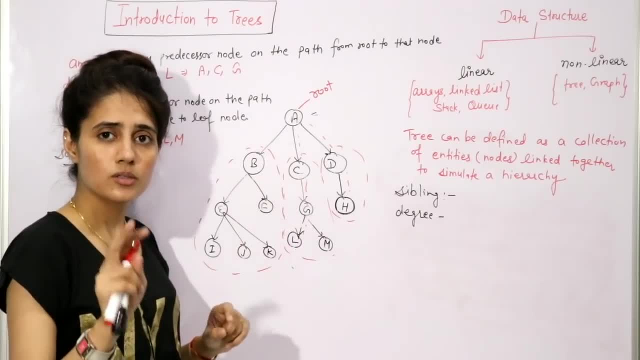 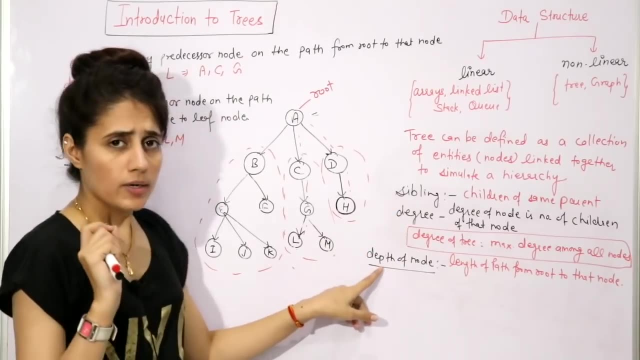 degree is 3.. So you can say degree of this tree is also 3.. So next is depth of a node. Here I have written sibling and what is Degree Right Now? depth of a node is what? C? The length of. 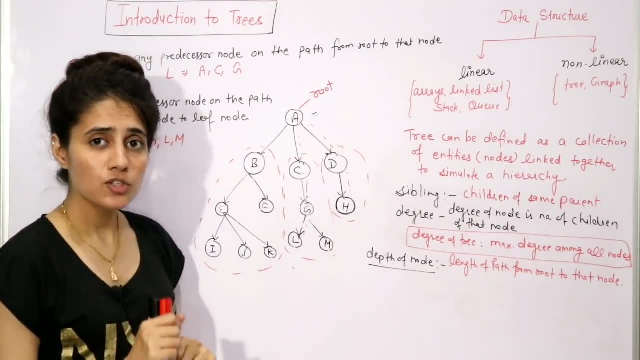 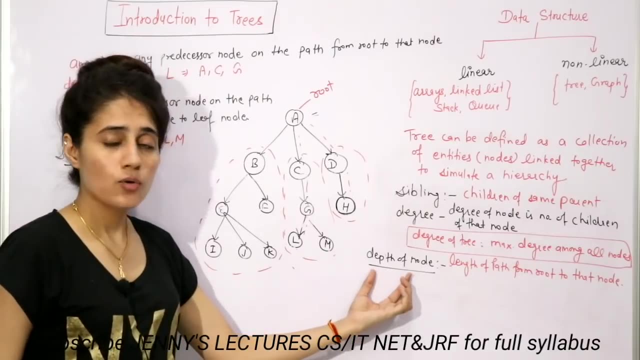 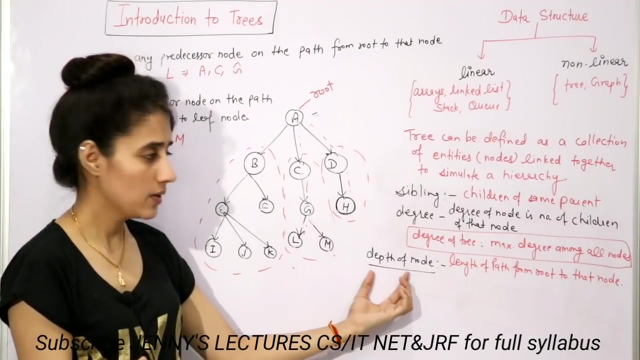 the length of the path. See now, path is what? As we have discussed, it is sequence of consecutive edges, Right? So in the simple terms, you can say what is depth of a node: Number of edges from root to that node. As simple as that. Right Now, if I ask you what is depth of F? Fine, So find. 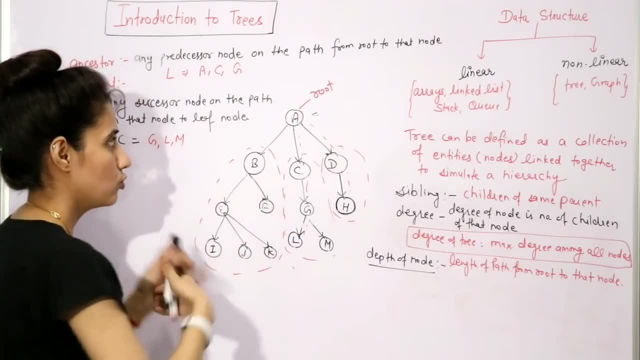 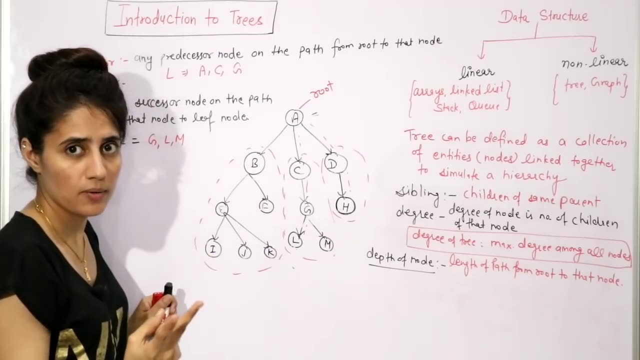 out the number of edges from root to this node. So root is A Number of edges from root to this node is what 1 and 2.. So depth of this is what 2.. Simple Right Now. if I ask you depth of J, Find out the. 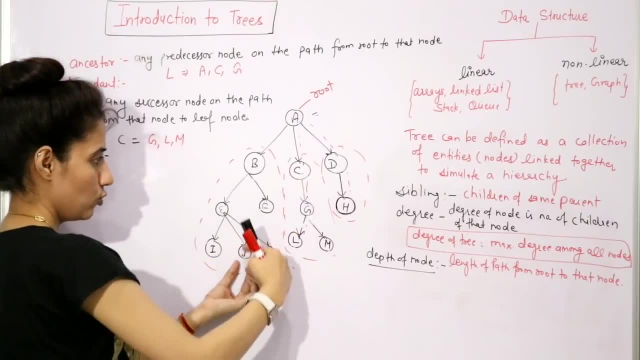 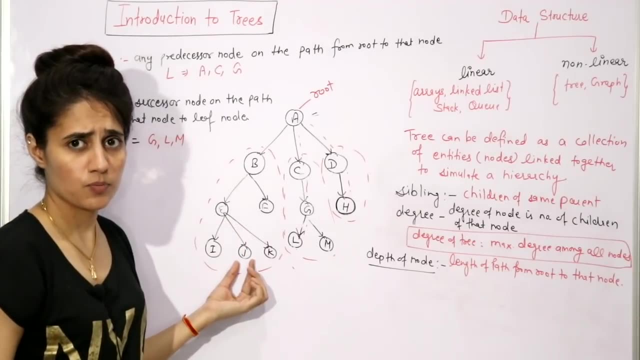 first of all, path from root to this node is this one, this one and this one. Number of edges are 1,, 2 and 3.. Just count the number of edges from root to that node. So this is what This depth. 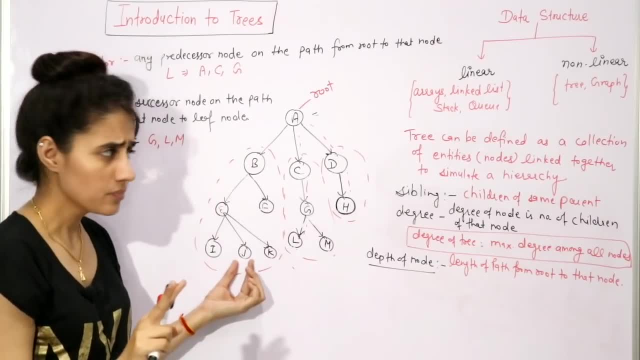 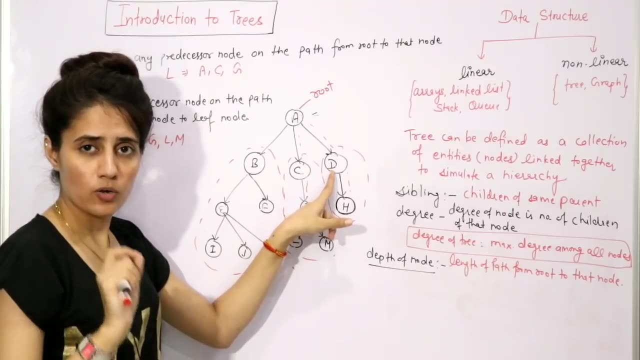 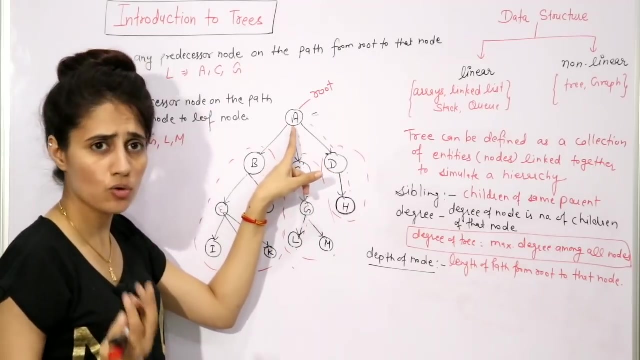 of J is what 1, 2 and 3 only Right. Depth of D is what Only one edge I have from root to this node, That is 1 only. Now what about depth of A? That is 0.. Because from root to A, A is only the root node, So there is no edge from root to this one. 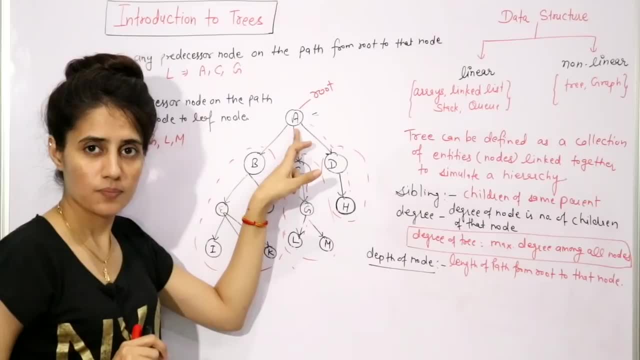 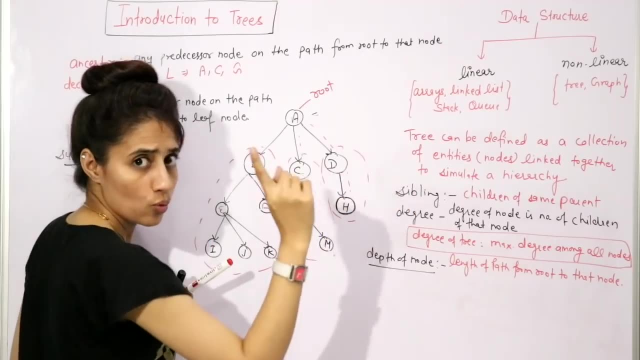 So the depth of root node is what? 0, always Right. So here you can say: the depth of this one is 0.. Depth of B, C and D is 1.. Depth of E, F, G, H: at this level. So this is what This is. 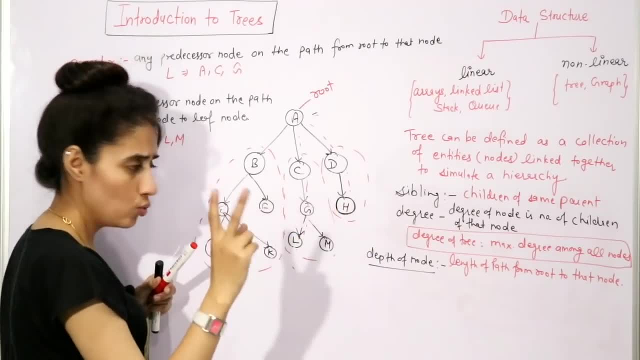 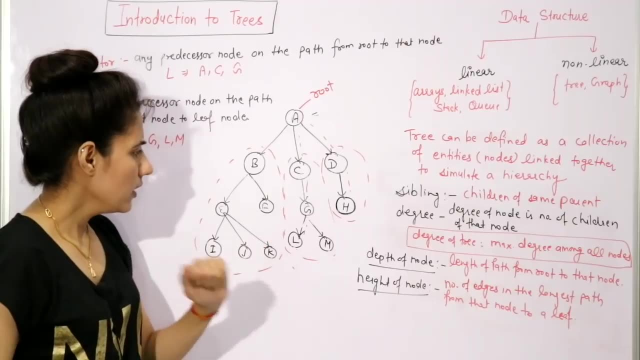 level. Depth of all these 4 are what? 2.. Depth of all these 5 are what 3.. Now, next is height of a node. See if I ask you what is height of G, Right? So height means from here, from bottom. 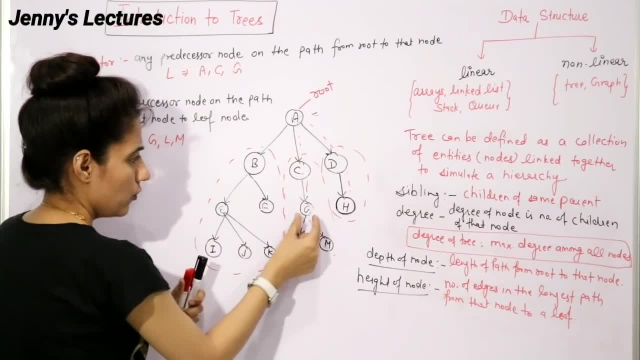 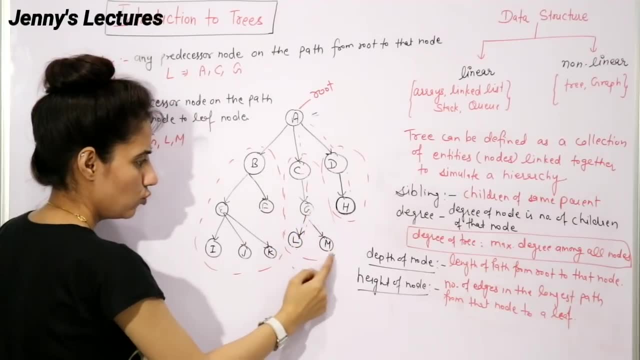 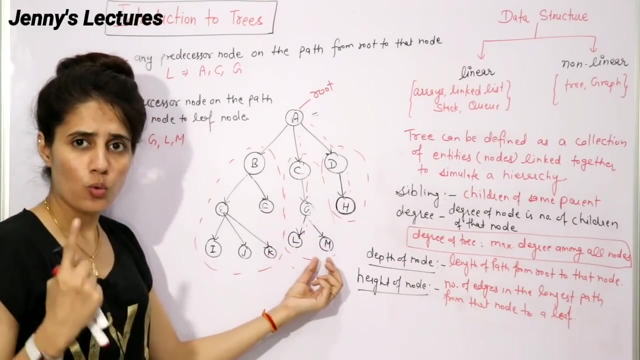 we will calculate the height. So from G you need to check out the path to its leaf node. G is having 2 leaf nodes only. So path is what? G to L, G to M, Both are having how many edges? 1. Right, Same edges. So the height of G is what? 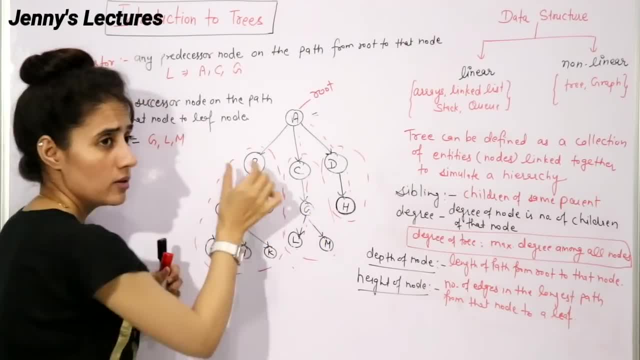 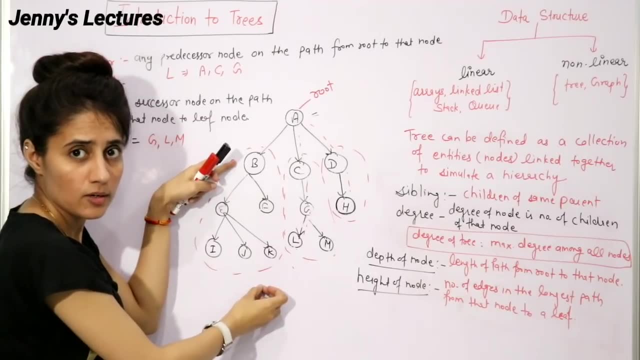 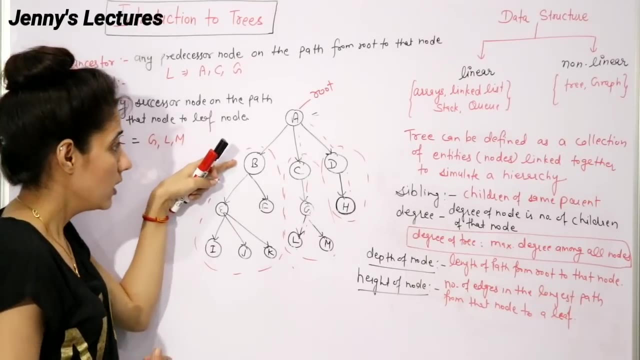 1. Now if I ask you height of B, just find out the path from that node to its leaf node Right, Or you can say to its deepest leaf node, Or you can say the longest path. you have to find out Right. So now, from B, see the leaf node are F also, but the path is G to L, G to M. 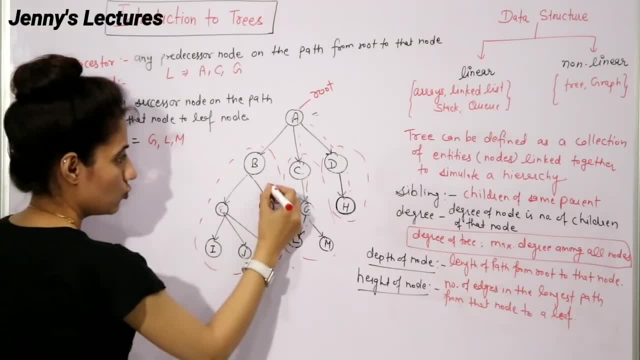 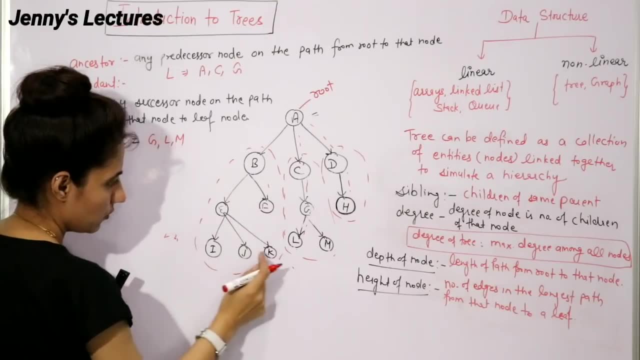 Path is having only 1 edge. So this is 1 edge, From B to I: 1,, 2.. 2 edges are there From B to J. we have 1,. 2 edges are there From B to K. also, we have 2 edges, And here I have 1.. So 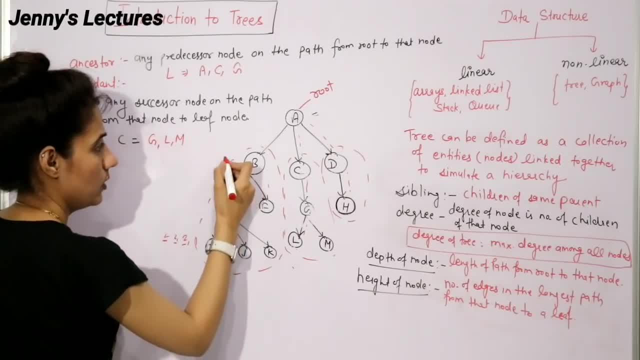 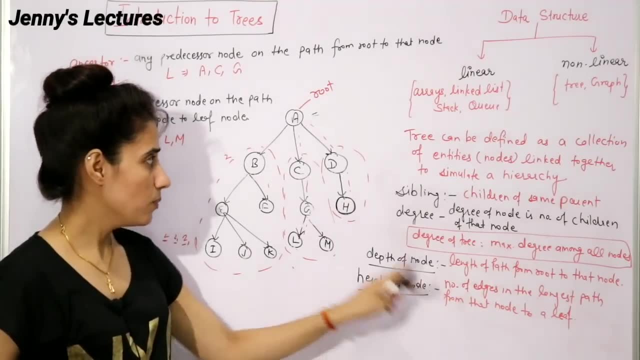 the maximum is what 2 only. So the height of B is what 2.. Right, So you have to find out the number of edges in the longest path from that node to a leaf node. Right, The longest path you need to. 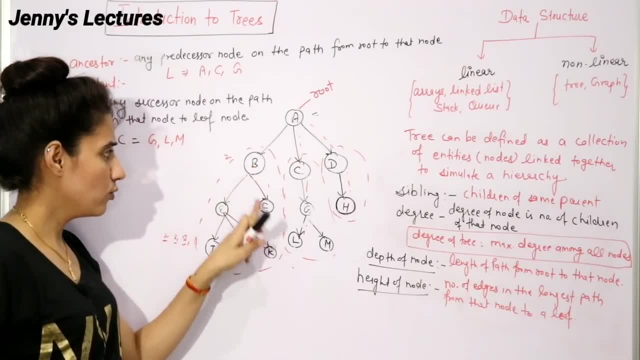 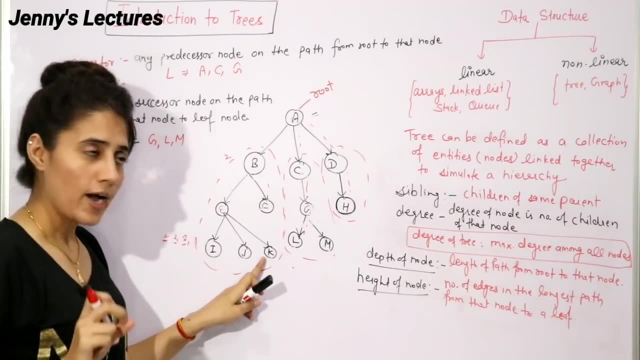 take care, It's not like that. It is also leaf node, So the height of this can be 1. No, Because the longest is what? 2. Longest path is what? 2. Having 2 edges. So the height is that one. 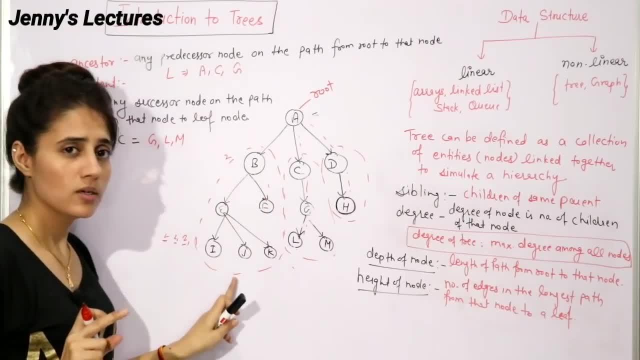 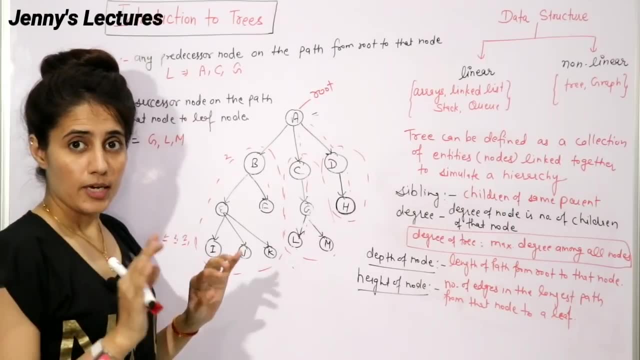 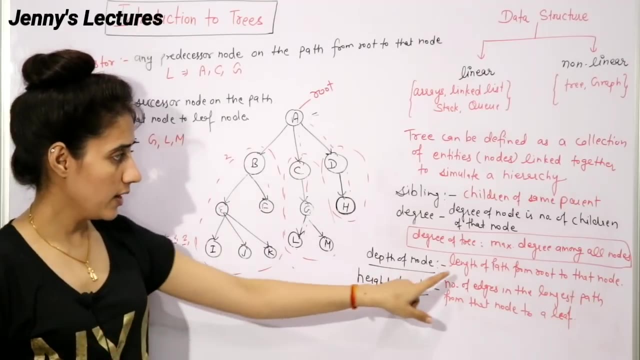 Right, The maximum distance we will take from that node to its leaf node. Now see: the height and depth of a node may or may not be same. Here you can take example of B. only Height of B is what. 2. Depth of B is what Depth we will always. 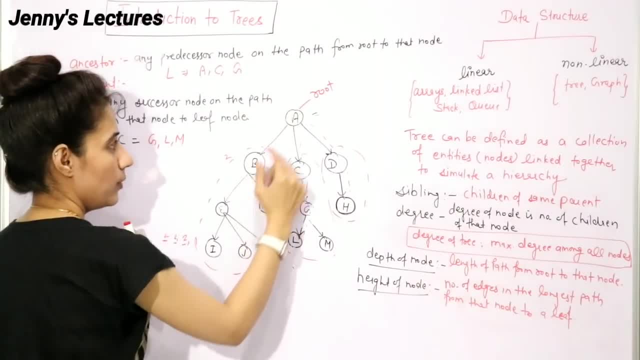 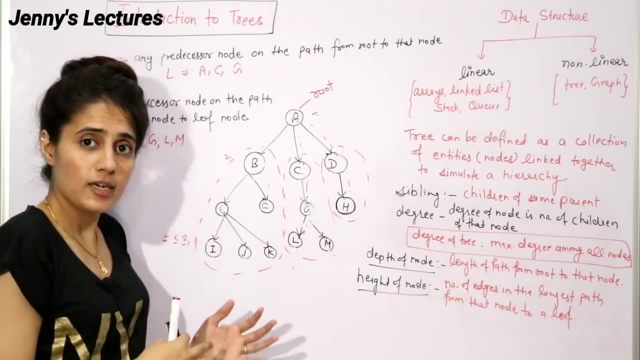 check from root to that node, So from root to B. number of edges are 1.. So depth is what 1. But height is 2.. Right, But may be. sometimes height and depth of a node may be same, So it may. or 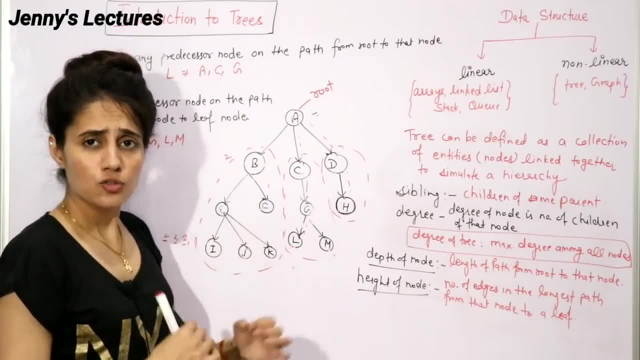 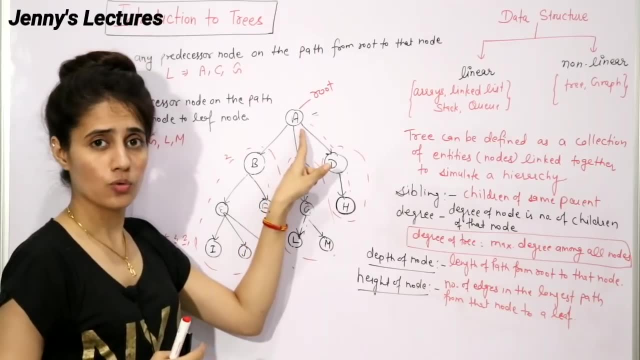 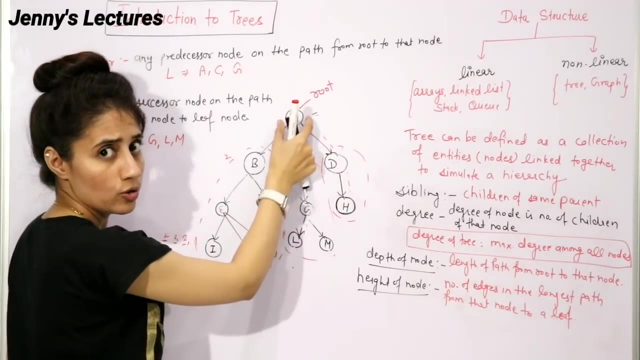 may not be same Right Now. height of a tree is what Height of this tree is equal to height of the root node. What is height of this root node Height? how you will find out, Find out the path, longest path from this node to its leaf. So all are these are leaf node of A, But the longest. 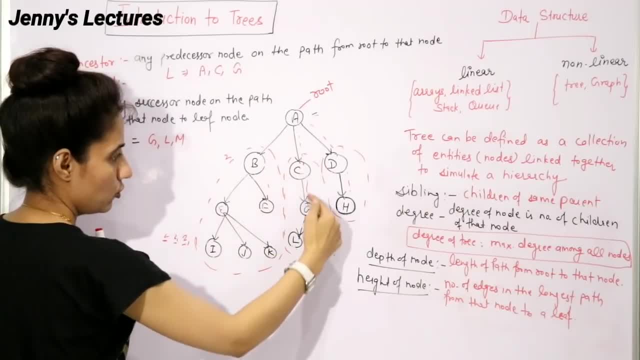 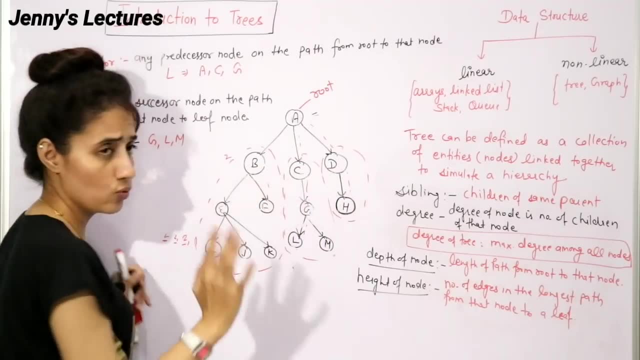 path is considering how many edges? I guess 1,, 2, 3.. This is also 1,, 2 and 3.. The longest is 3.. This is 1 and 2.. This is also 1 and 2.. So the height of this one is what? 3. Height of root. 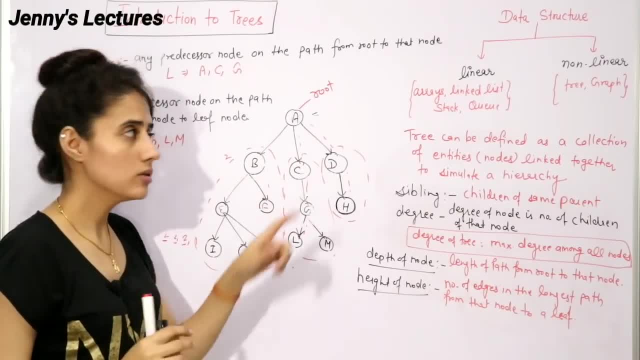 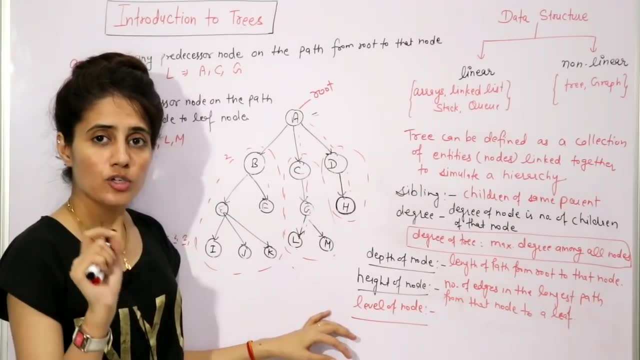 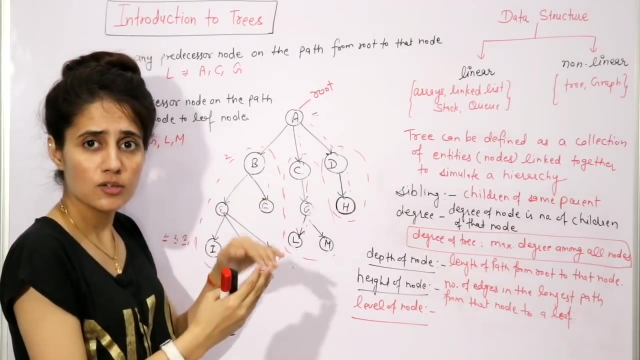 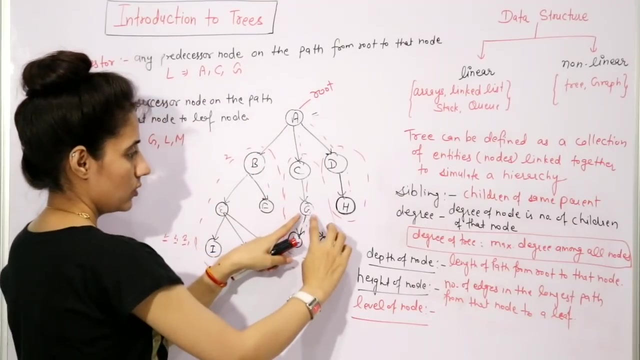 node as well as height of this tree. is what? 3 only Right Now. what is level of a node? See, level of a node is also the distance from root to the given node Right. Or you can say number of edges from root to given node in that path. So if I ask you, level of G, So the distance. 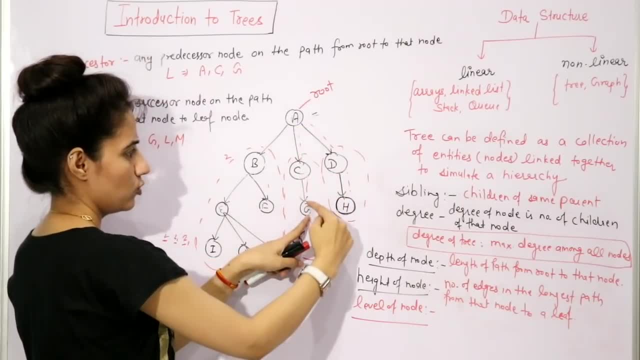 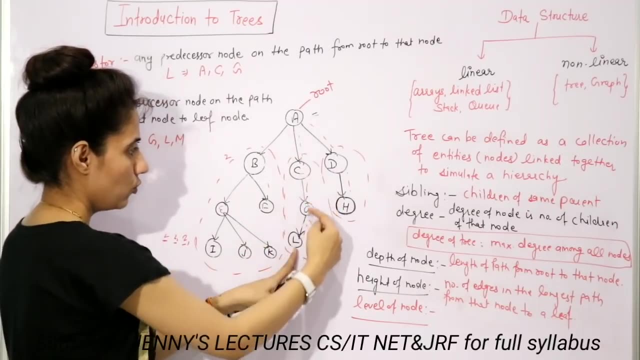 of this G from root is what? The path is this one and this one? How many edges are there? 1 and 2.. So the level of G is what? 2.. Level of L is what? 1, 2 and 3.. Or here you can say: 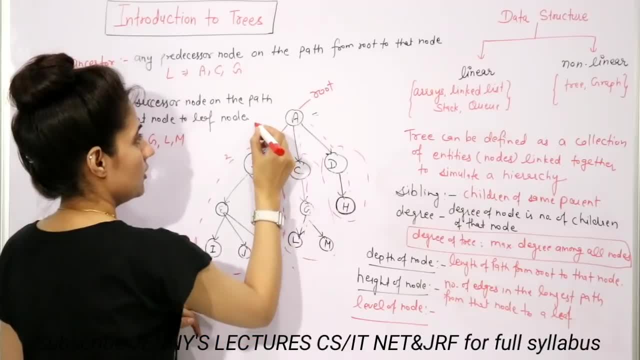 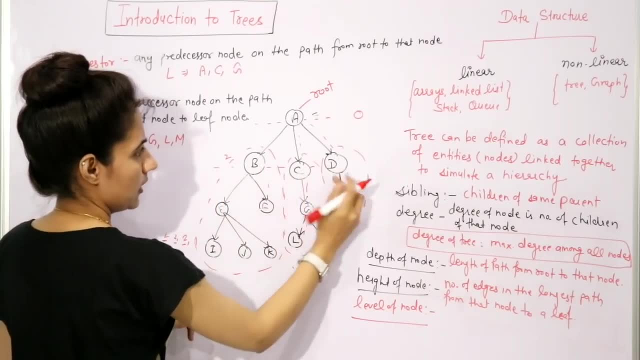 each hierarchy or each step is known as level. See, this is not. this is known as 0th level. Next level is this one: B, C and D. This is what Level 1. This is known as level 2.. This is known. 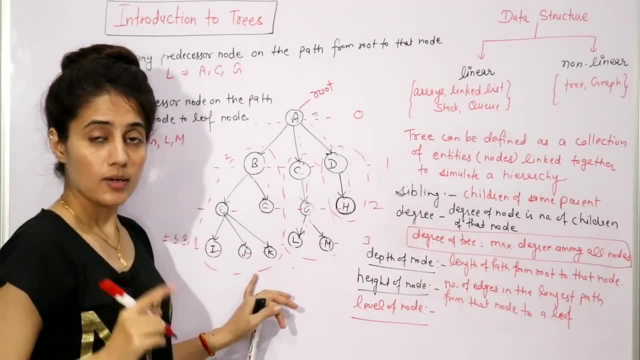 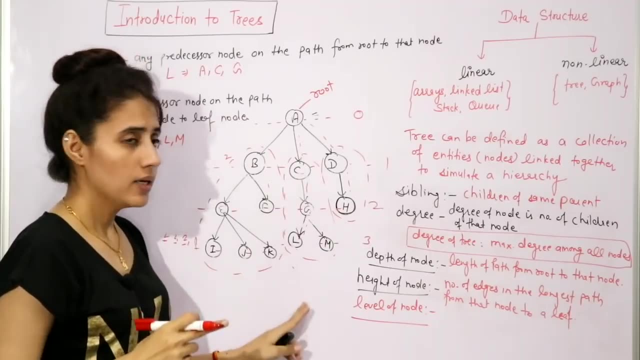 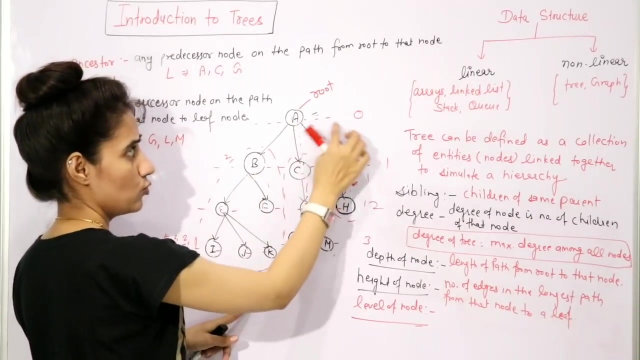 as level 3.. Right, And this level of a node is always equal to depth of the node And as well as level of a tree. See here, the level of this tree is what: 3.. How many hierarchy? What? This one, this one, this one and this one? But this is what? 0th level and 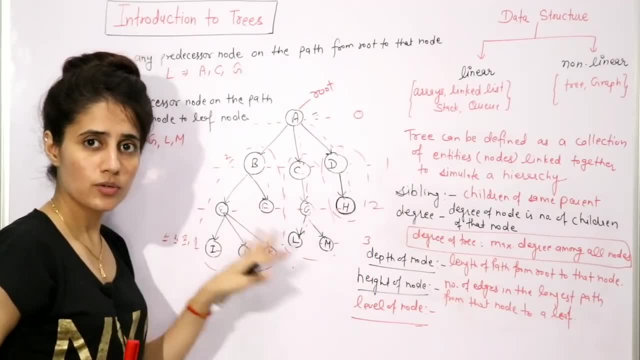 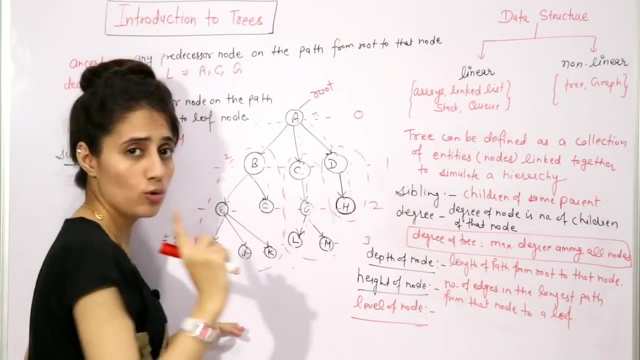 the maximum is 3.. So the level of this tree is what? 3. See, you can say level of tree is equal to height of the tree. Height of this tree is also 3. How you will calculate the height Number of? 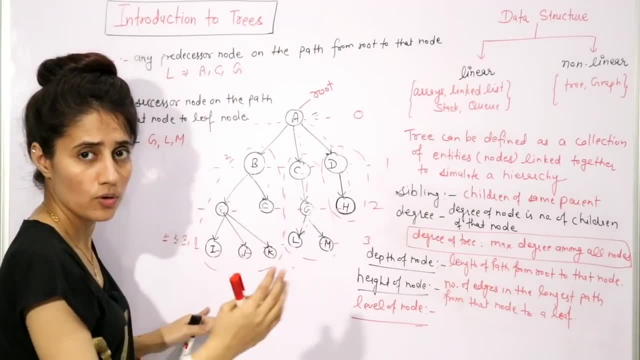 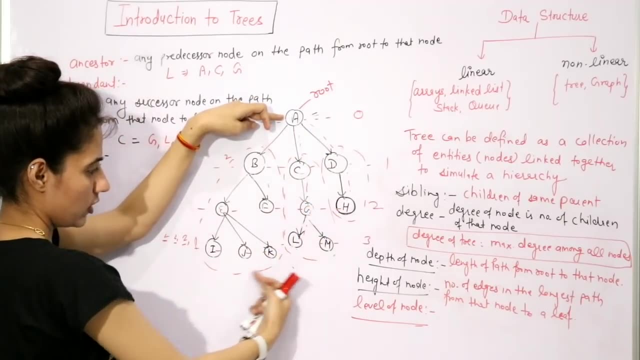 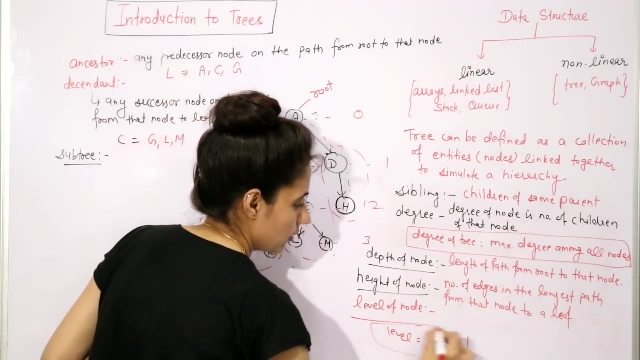 edges in the longest path from that node to leaf node. And height of this tree is what Just find out. height of the root node, Height of the root node is what 1, 2 and 3. The longest path, 3 edges. So you can say level of a tree is equal to height of a tree, But level of a node is not. 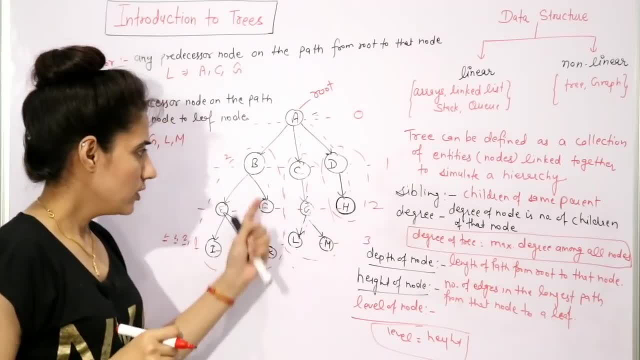 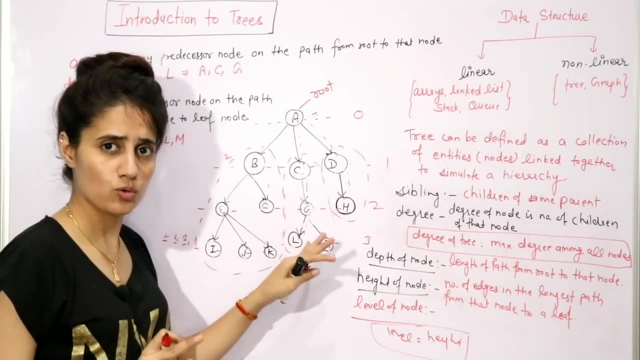 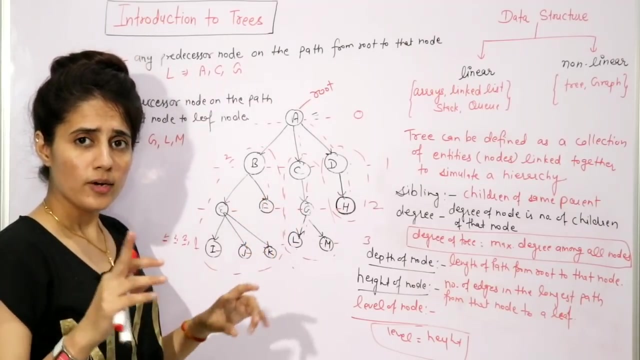 equal to height of a node, And level of the tree is also equal to depth of the tree And level of a node is equal to depth of a node. Right, You can check out this also with this example. Fine, Now I guess I have discussed all the terminologies used in the tree Right. One important point is: 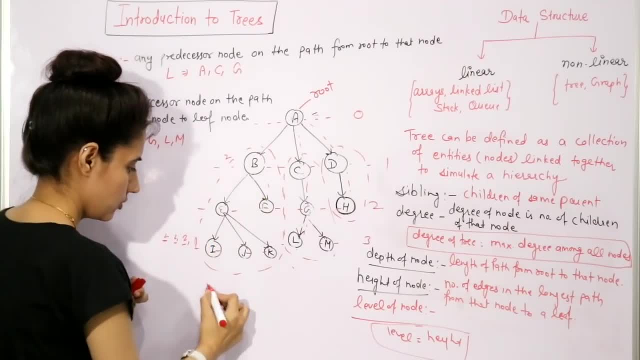 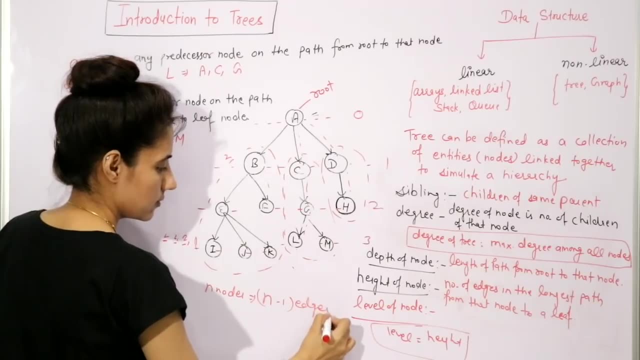 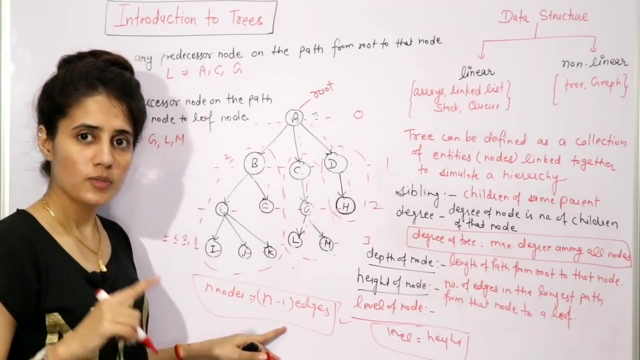 if in the tree I have n nodes Right, In that case there should be n minus 1 edges. Here also you can count the number of nodes as well as the number of edges. That is the condition. Right Of a tree, n nodes means n minus 1 edges should be there, And if you will add one more edge, 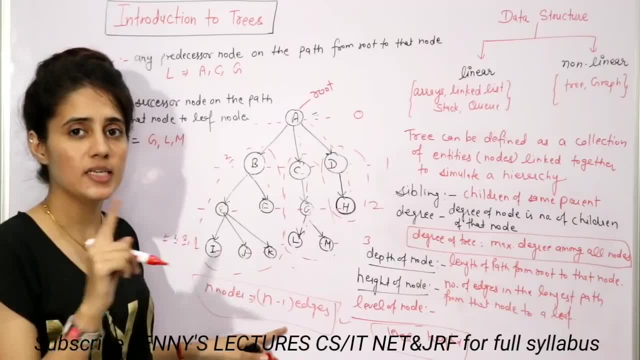 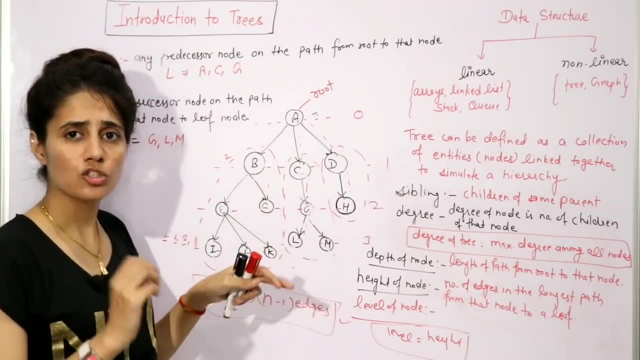 it means it will form a cycle, But in a tree we cannot have any cycle. It should be a cyclic. Right Now, how you are going to actually implement this tree. See, this is just a logical representation of a tree. Obviously we cannot. 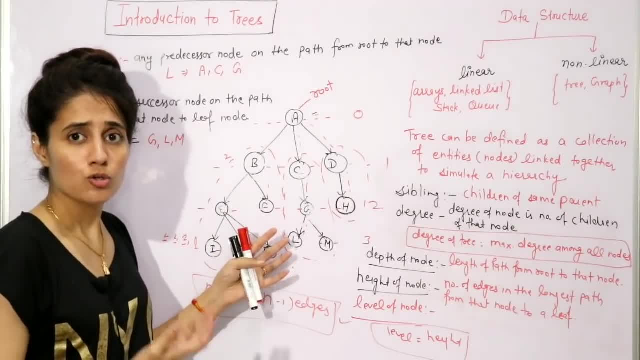 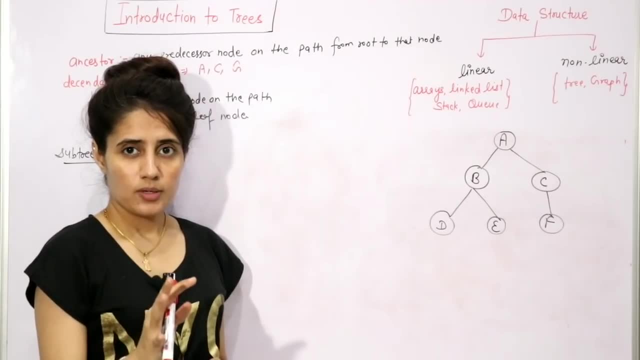 represent a tree in the memory, something like this: Right, So how we are going to represent that this tree into the memory. See, See now here. basically, we will discuss about binary trees. It means a tree can have at most two children. So how you are going to represent this binary. 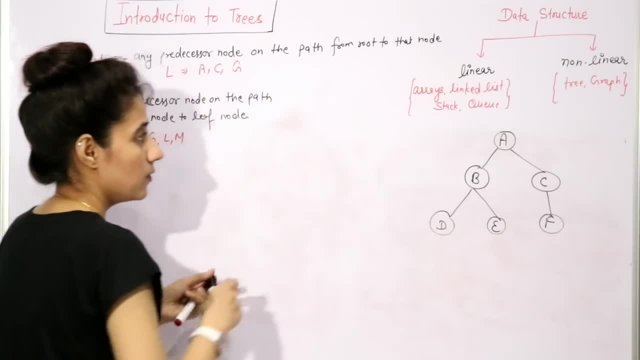 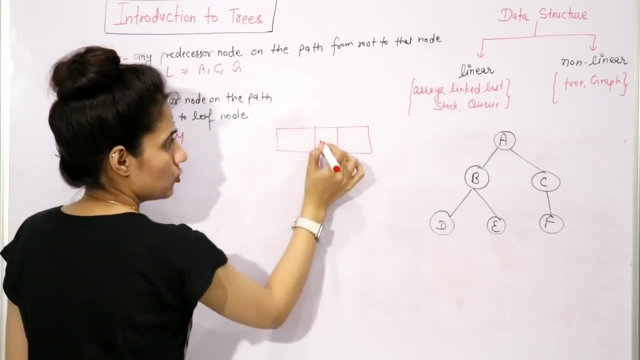 tree, actually How you are going to implement this one. See, these are nodes, So how we are going to represent a node here Dynamically. obviously we are going to implement a node here. We are going to create a node, So this is what a data part which is containing this data, as well as 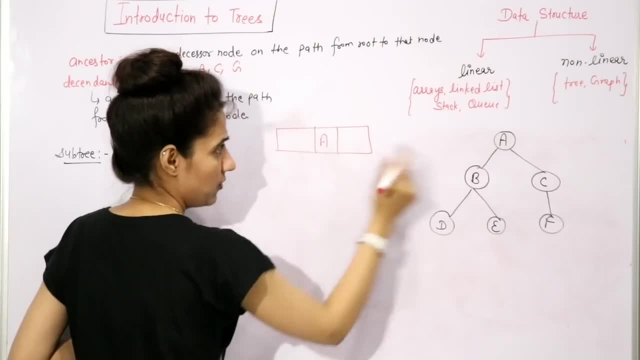 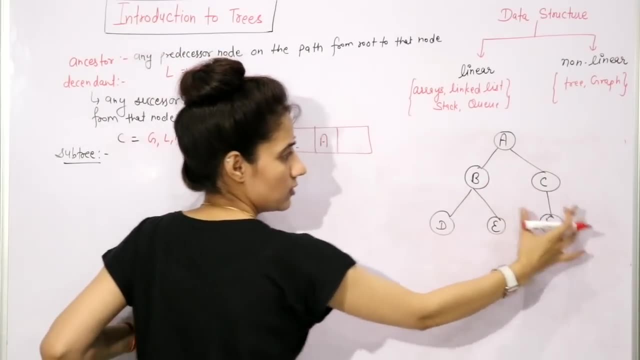 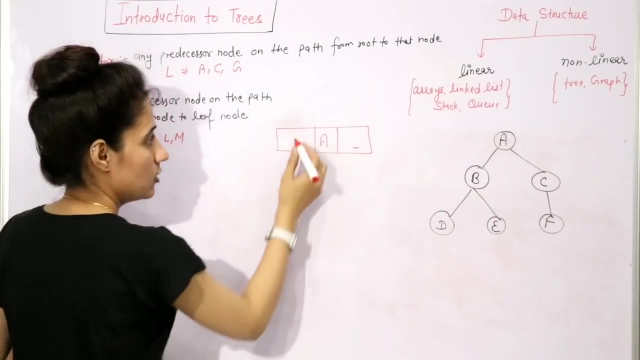 two links are there. One is link means one link, left link. This will contain address of the sub, this left subtree. This is going to contain address of this subtree, Right, Or you can say: root of this subtree and root of this subtree. So two links would be there. This is what you. 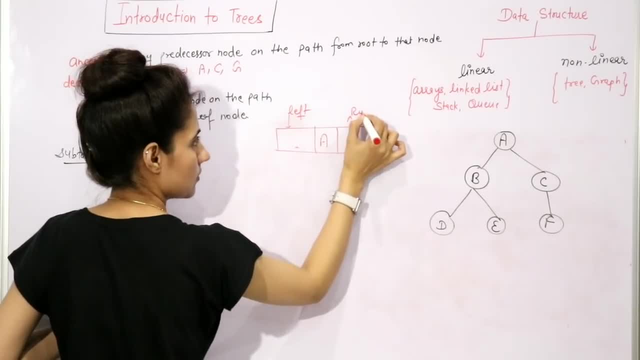 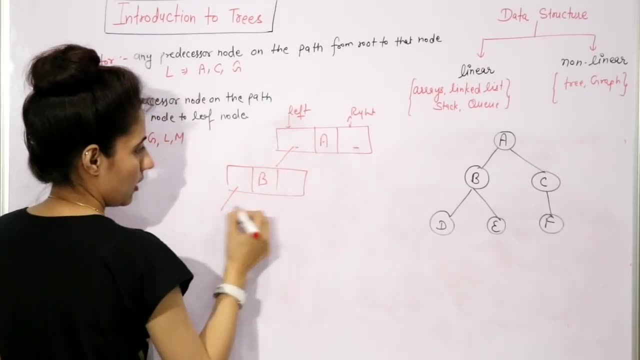 can say left link or this is what right one Right Now. here also we are going to create a node. So we are having what We are having: data B. B is also having two links. So here we have what D and 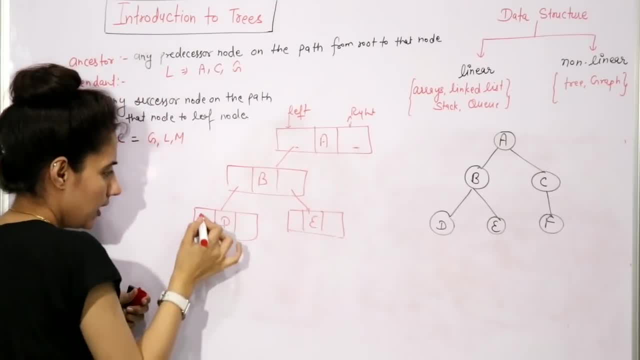 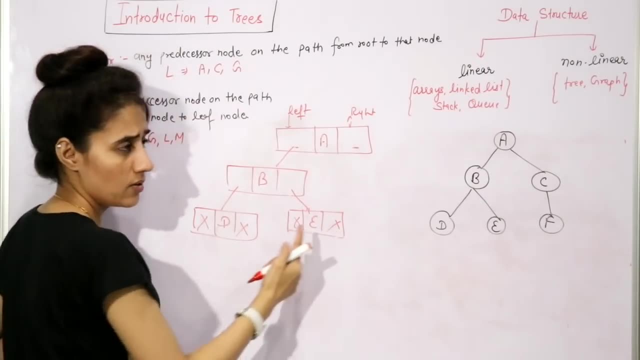 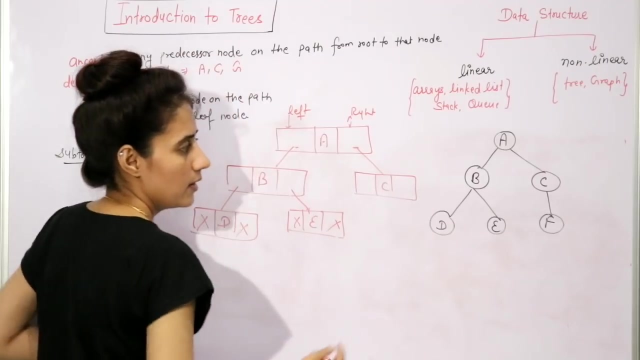 here we have what E, But here we don't have anything, because D is not having any child node, E is also not having any child node. So here in the left and right link we will store null only Right. Here we have C Right And in C suppose this is what The right. 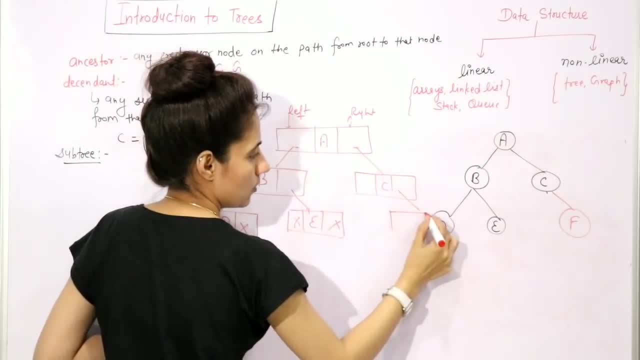 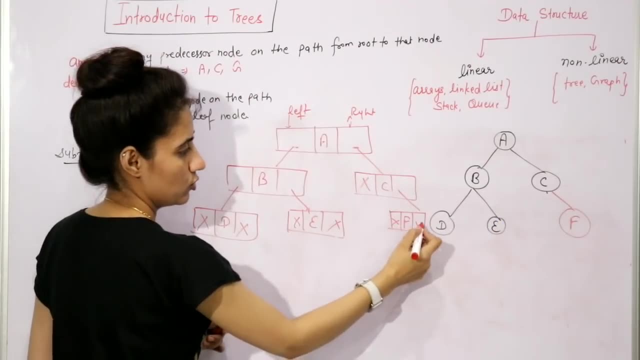 Child Right. So here I have F, But in the left I don't have anything because there is no left child. So here you will store null, Here also we will store null. This is how we are going to. 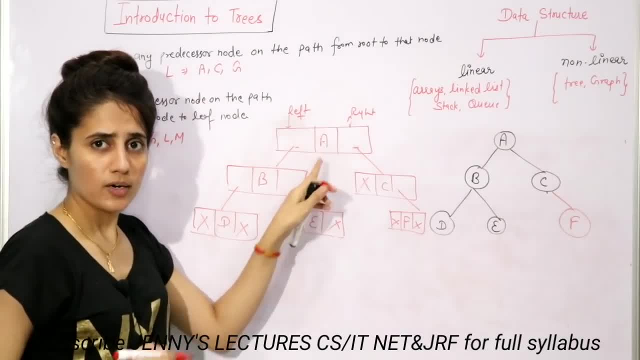 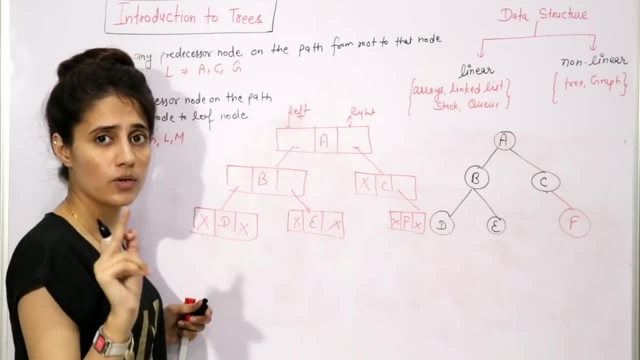 actually implement the tree. These are nodes Right Now- how you will write down in the code, See how you are going to create this node. This thing we have already discussed when we were discussing the linked list. Obviously, we are going to dynamically create this node, So we are. 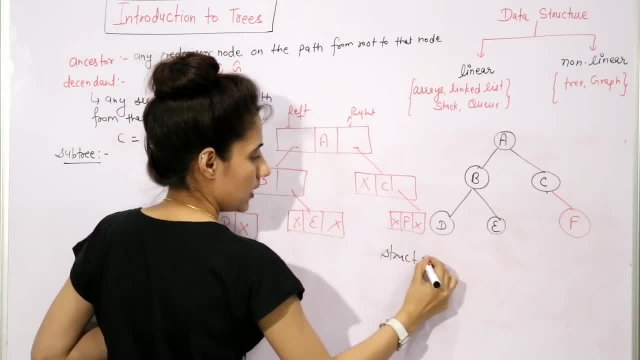 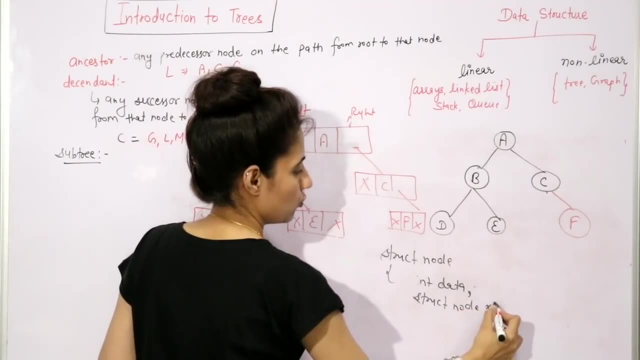 going to use what Struct? The name is what I am taking node, And here I am taking three parts. One is data part, Next is two links would be there, One is left and one is what Struct node- Historic Right link. 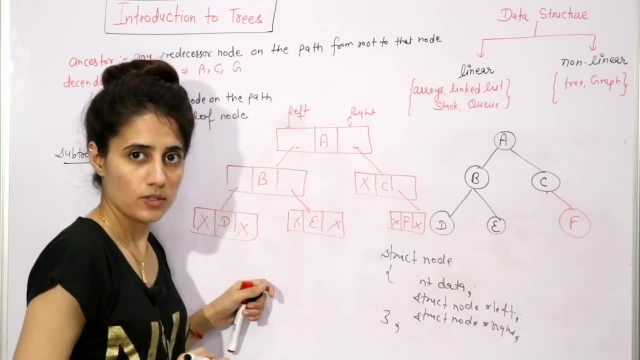 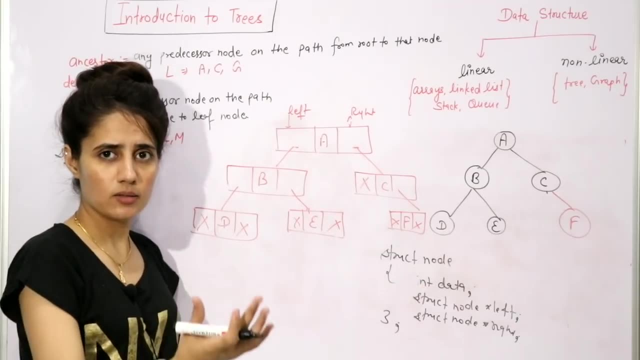 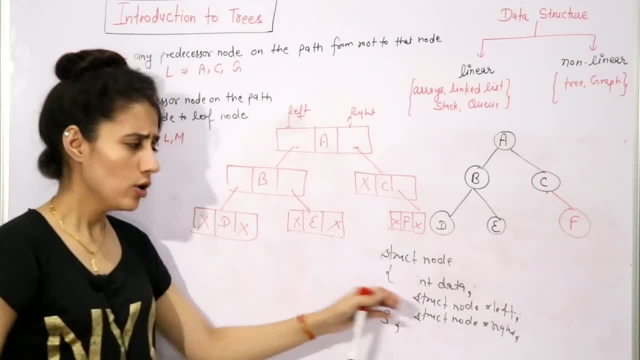 basically, you can consider: here I am having 1,, 2,, 3,, 4. Right. Or you can write here: care also, float also as you wish, Or you can take string also. Fine, That is not a big deal. So now what? 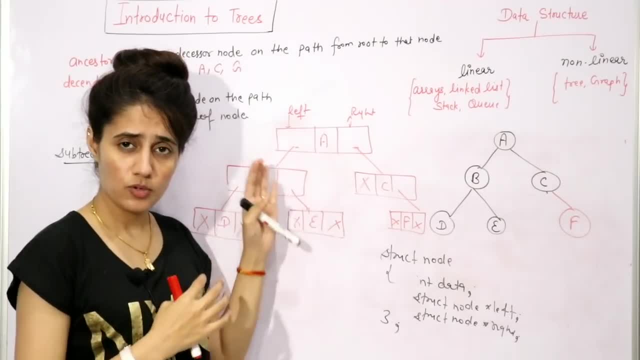 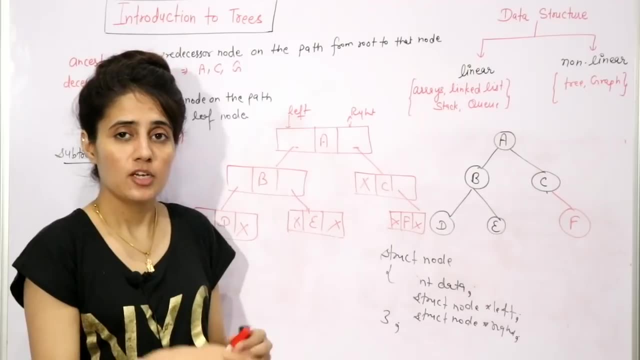 are the applications of pre data structure? See, obviously we have discussed tree is going to store what Hierarchical data. So it is going to, you know, implement a that file system. In file system also we store data something like this: Here we have directory, Then we have sub. 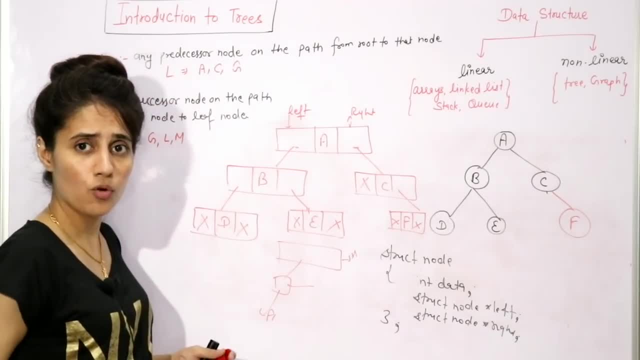 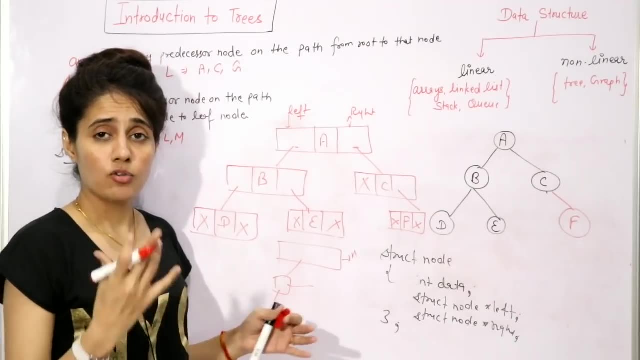 directories, Then we have file. So this is what A hierarchical form. So trees are going to store- what A hierarchical form. So this is what A hierarchical form. So this is what A hierarchical to basically implement this model, That file system, Right In routing protocols. also, we are 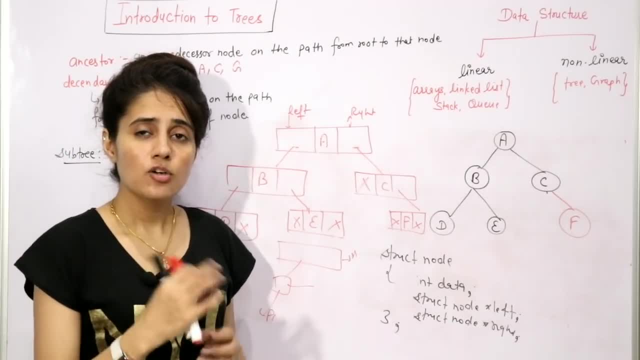 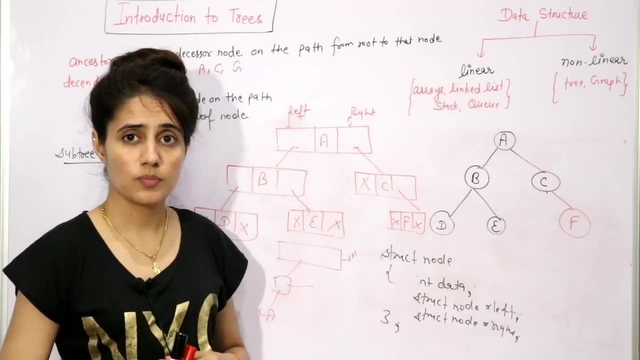 going to use tree data structure. Next application may be it organize the data for a quick search or insertion and deletion, Like you can say as a binary search. tree Heap tree also Right. So there are many applications of tree One by one applications also we will discuss in later videos. 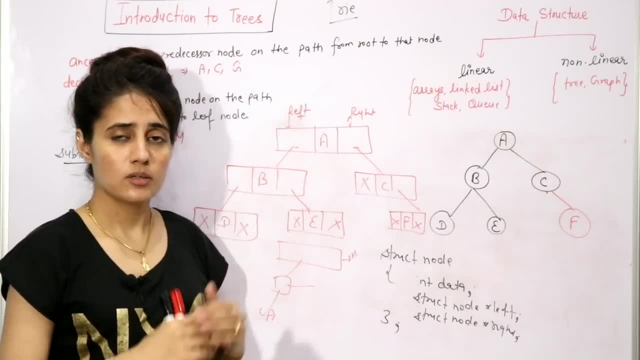 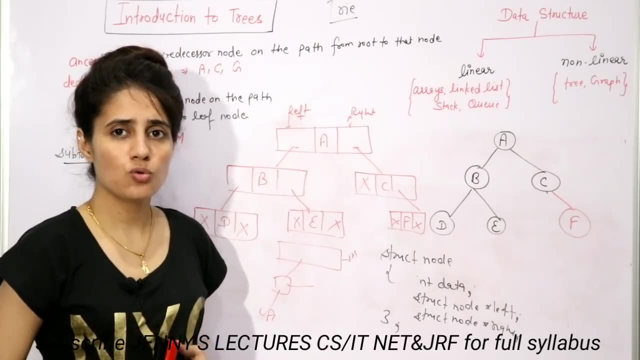 with the implementation. So now, in next video we will discuss types of trees. You know you can say brief introduction of types of trees, Binary, binary search tree, avial tree and all that. After that we will discuss those trees in details. So I will see you in the next video. Till then, bye, bye, Take care.